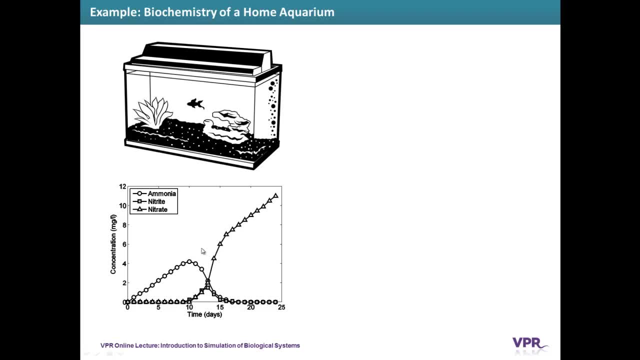 So here I am showing data on levels of three compounds- ammonia, nitrite and nitrate- in a newly established home aquarium. So these trends- a buildup and a decay of ammonia, followed by a buildup and a decay of nitrite, followed by a buildup of nitrate- are familiar to fish keepers. 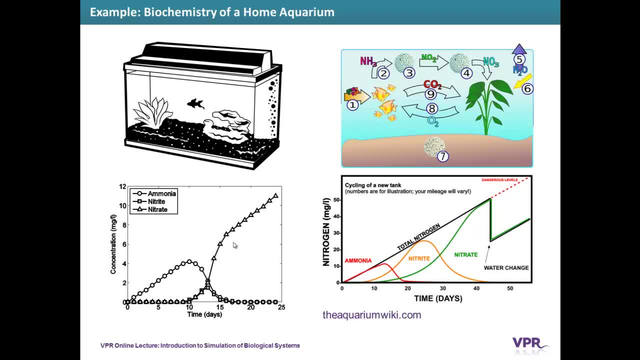 And you can easily find illustrations of these phenomena at places like theaquariumwikicom, which is where I got these figures. What is happening here is that fish in the fish tank excrete ammonia, which is oxidized to nitrite, and nitrite is oxidized to nitrate. 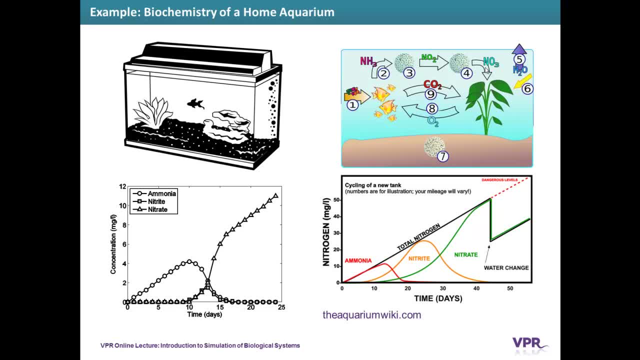 And these oxidation processes occur in bacteria, particularly in the aquarium filter In a brand new aquarium setup. populations of bacteria have yet to be established, And so what you see happening here early on for the first week or so is that ammonia is building up, and these products- nitrite and nitrate- have not started to build up yet. 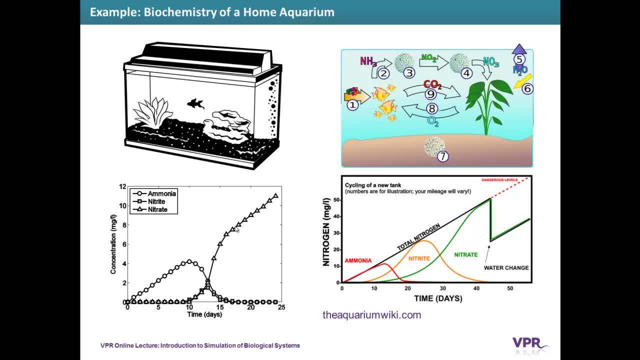 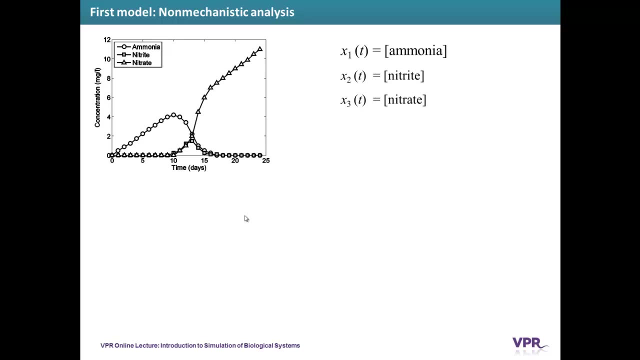 until the bacteria grow in substantial enough quantities to manage these waste products. So, essentially, this is the phenomenon that we are interested in understanding, and these are our data. So what can we do? So the first thing we do is a bit of bookkeeping. 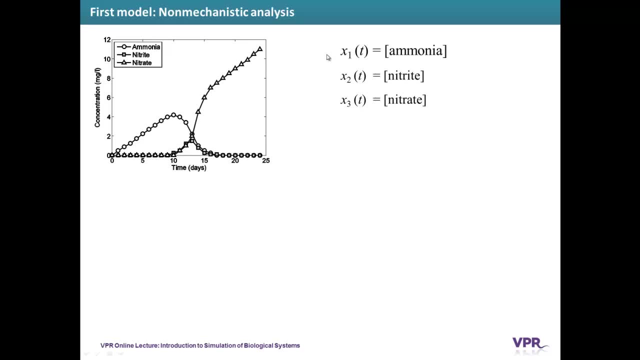 We assign variable names to the concentrations of interest in the system. So, for example, we can assign the variables X1, X2, and X3 to represent ammonia nitrite and nitrite. This might seem like some unnecessary abstraction and potentially confusing. 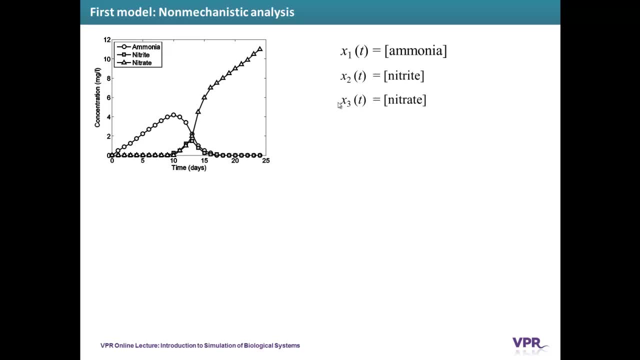 However, it turns out, in my opinion, that it's easier to work with X1,, X2, and X3 that carry around these full names: ammonia, nitrite and nitrite. Don't worry, I'll keep reminding you of what X1, X2, and X3 refer to, so hopefully there will be no confusion. 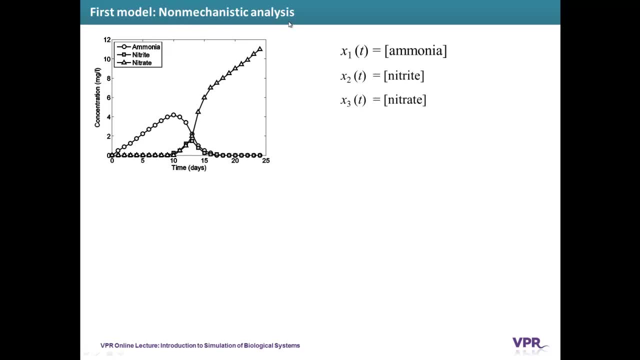 Now I refer to our first model of this system as a non-mechanistic analysis, And what I mean by that is that we are going to analyze these data without any attempt to capture the mechanism of how X1 converts to X2, and how X2 converts to X3. 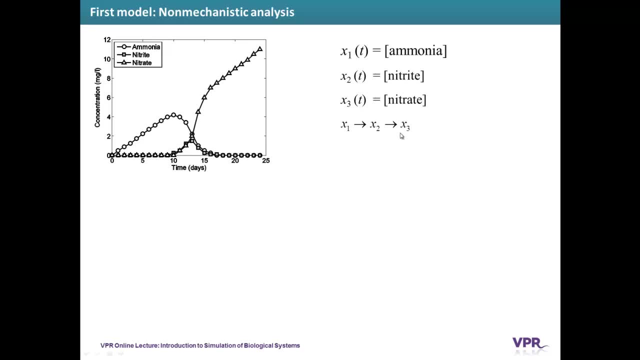 Now you could argue that this phenomenon of X1 to X2 and X2 to X3 is a mechanism, and that's fair enough. We don't want to get bogged down in terminology, and you'll see in the second half of this lecture what I mean by a mechanistic or maybe a more mechanistic model. 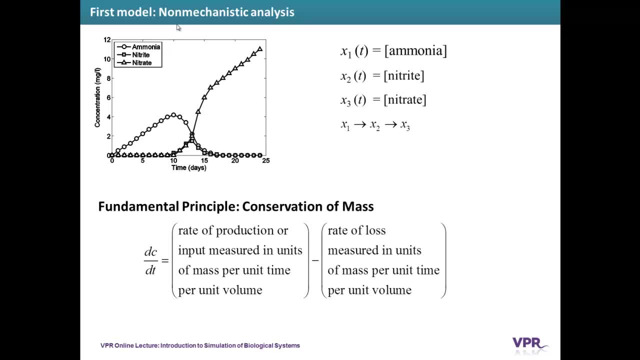 In any event, all of our analyses will be based on the fundamental principle of the conservation of mass, which can be written down in equation form like: so: So what we're saying in this equation is that the rate of change of some concentration is simply the rate of production or input of mass into the system, measured in units of mass per unit time per unit volume, minus the rate of loss, measured in units of mass per unit time per unit volume. 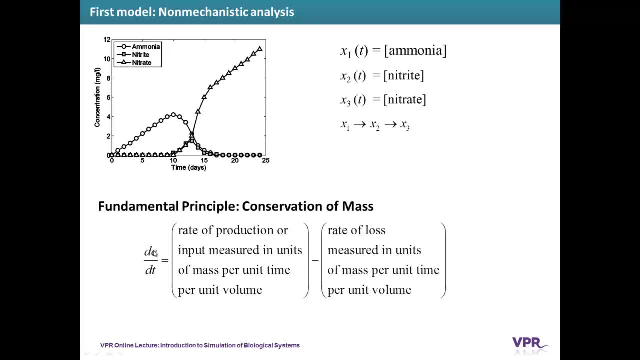 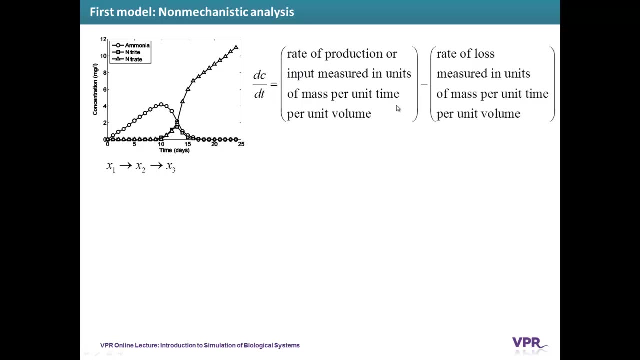 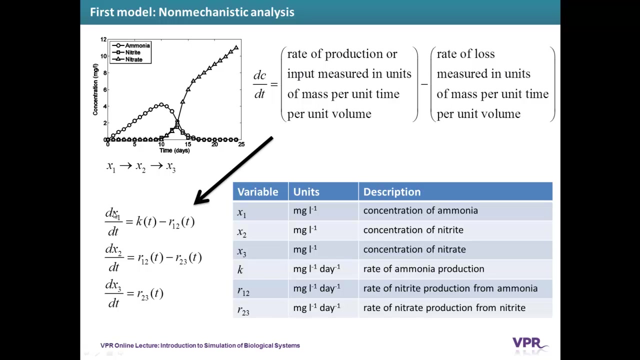 So this is simply a statement of what you have in. the rate of change of what you have in the system is equal to the rate at which you put in mass You put stuff in, minus the rate at which you're taking stuff out. So here is that generic statement of conservation of mass again, and translating that into equations for use. in our system where we have X1,, X2, and X3, we have a total of six variables to account for. 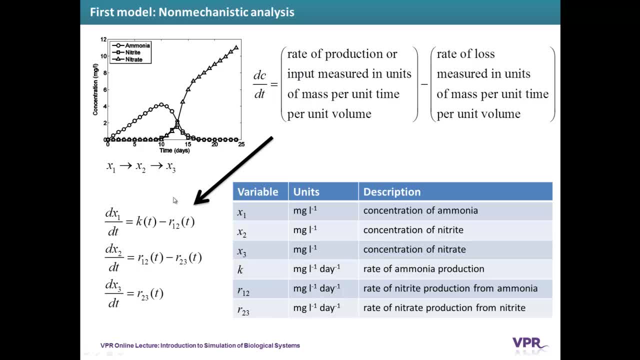 Three are our concentration variables. One is the input of X1 into the system, or the rate of ammonia production, which I'm denoting by K. and then we have these rates of conversions: R12, the rate of nitrite production from ammonia. 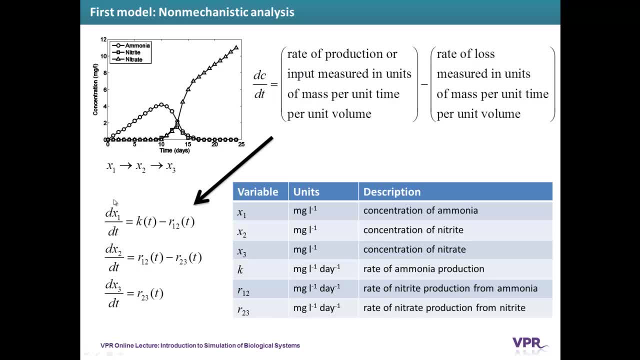 R23,, which is the rate of nitrate production from nitrite. So the rate of change of X1, or ammonia, is equal to the rate of input or production of ammonia, minus the rate of conversion of that ammonia into nitrite. 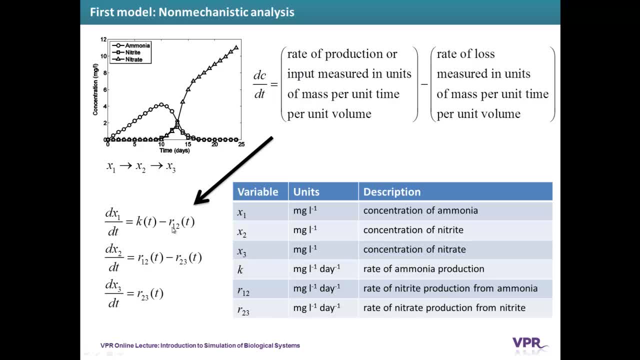 Our nitrite equation, dx2dt has this same term, this rate of production term, but where it has a negative sign in front of it in the ammonia equation, has a positive sign in front of it in the nitrite equation, because the conversion of ammonia to nitrite is a loss of ammonia and it's a gain of nitrite. 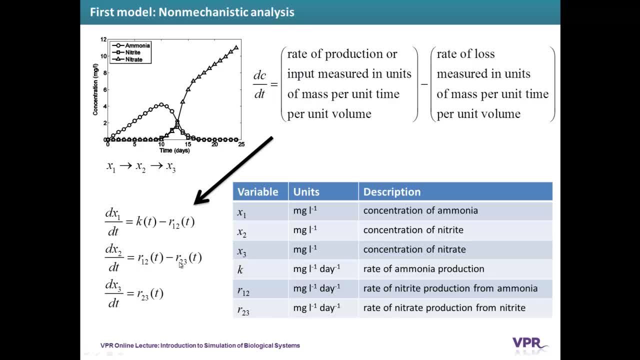 Similarly we have a loss of nitrite, which is the rate of conversion of species 2, nitrite into species 3, ammonia, And similarly this loss term appears as a gain term in our equation for nitrite. So dx3dt is equal to the rate of nitrate production from nitrite. 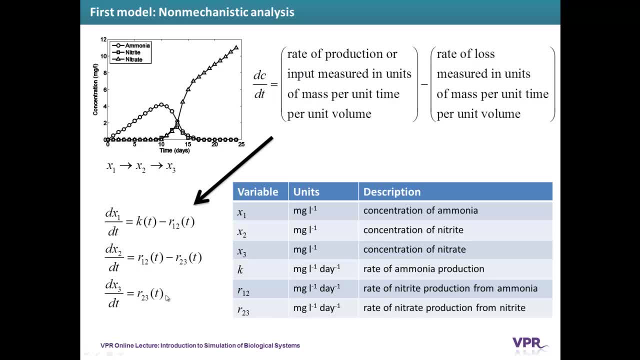 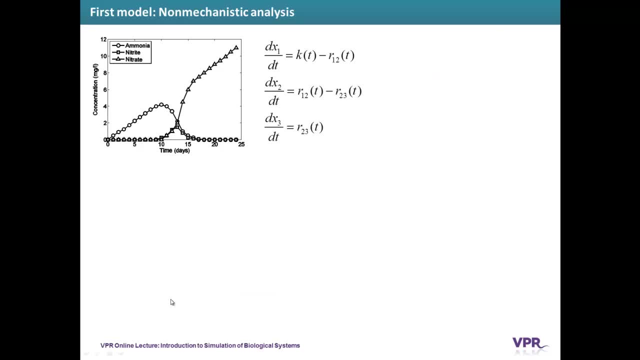 And in our system we have assumed that there's no way for the nitrite to disappear, so there's no loss term for nitrite. So here are those equations written again up here And in order to analyze our data and estimate what these rates are in this system. 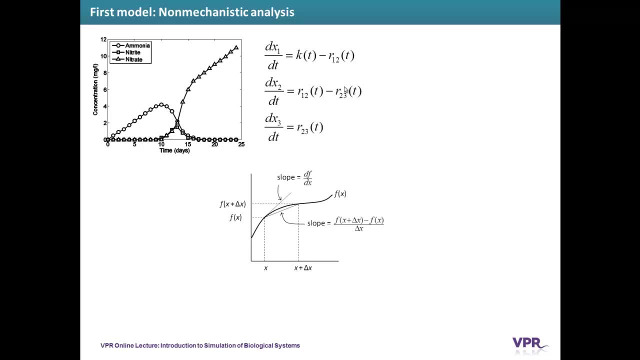 we're going to turn to a little bit of simple mathematics, And what I'm showing you here is something called a finite difference, approximation for the derivative of a function. So here I'm plotting some function, f, a function of a variable x, and the derivative of that function, df with respect to x. 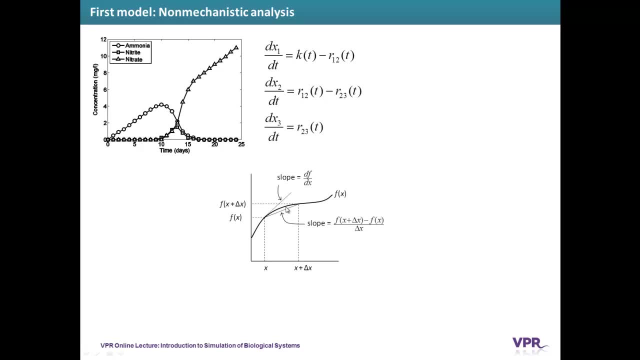 is the slope at any particular point x of this curve. Now we can estimate that slope over some finite difference in x as the difference between the value at x plus delta x and the value at x, So f at x plus delta x. 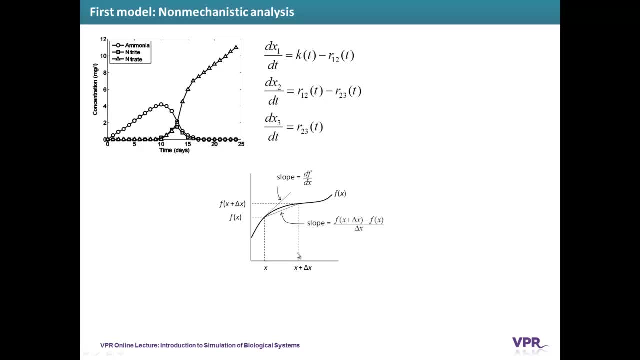 minus f at x, divided by the finite change in x delta x. So you can imagine that as this delta x gets very, very small, this finite difference slope approximates this continuous derivative df, dx, And that's the essential piece of mathematics which we're going to use to estimate these rates. 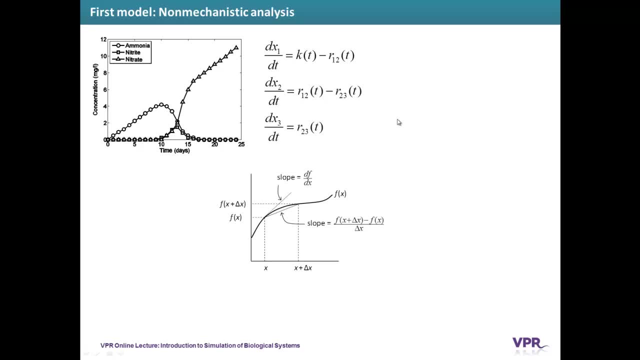 from this simple conservation model for our fish tank, Specifically the R23,. this production of nitrate rate is equal to the dx dt for x3.. We estimate that R23 as a finite difference approximation for the derivative of x3, and here I'm using a centered difference approximation. 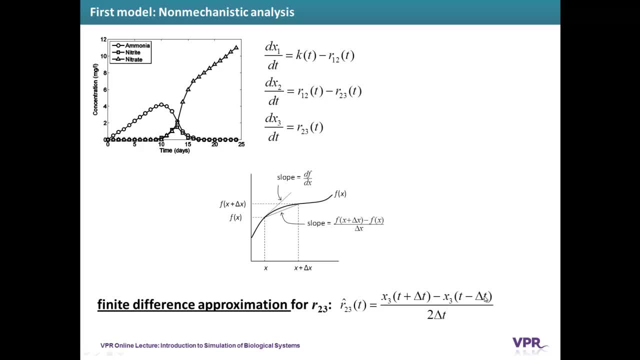 x3 at t plus delta t minus x3 at t minus delta t and we're dividing by the width of the time interval, which in this case is 2 times delta t. I put a little hat on this R23 to indicate that this is the numerical estimate. 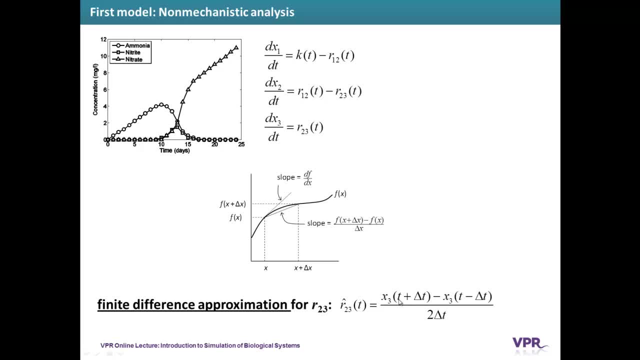 of this rate from these data, measured at times t plus delta t and t minus delta t. So that's our approximation for R23.. Given our approximation for R23, we can look at our second equation and the R12,, the rate of conversion of ammonia to nitrite. 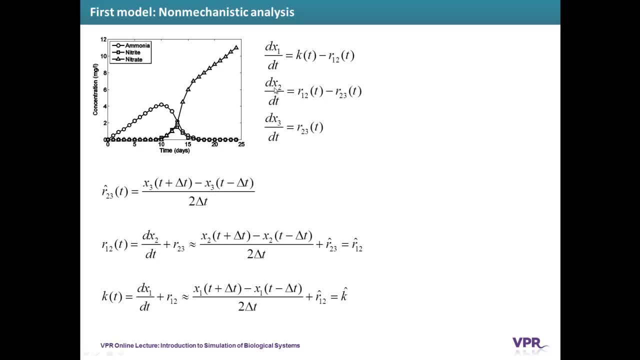 we can approximate as the finite difference, approximation of dx2 dt plus R23, which we've already approximated. So, just doing the same sort of thing, we have the finite difference approximation for R12, with our little hat. Similarly, our rate of ammonia production. 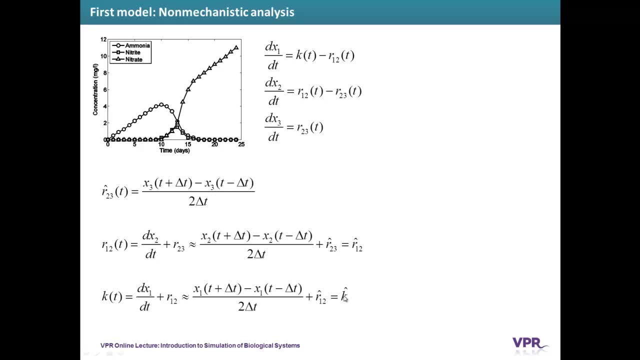 k hat. the estimate of k is equal to the finite difference approximation of this derivative, dx1 dt plus our estimation of R12.. R12 has a little hat on it. So what these equations do is they allow us to directly estimate all of the rates in our 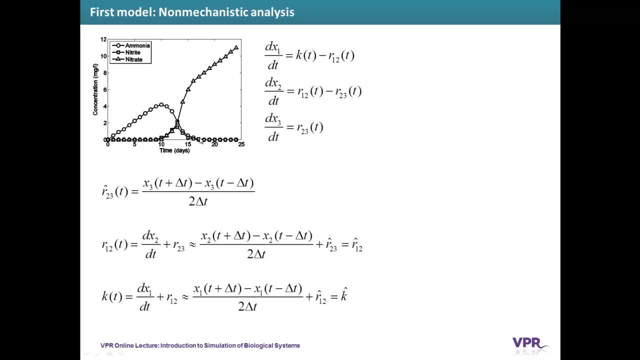 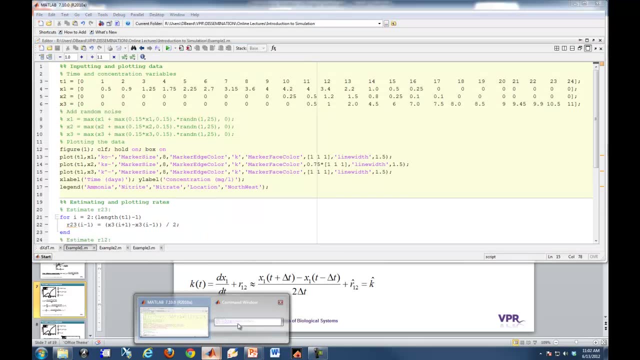 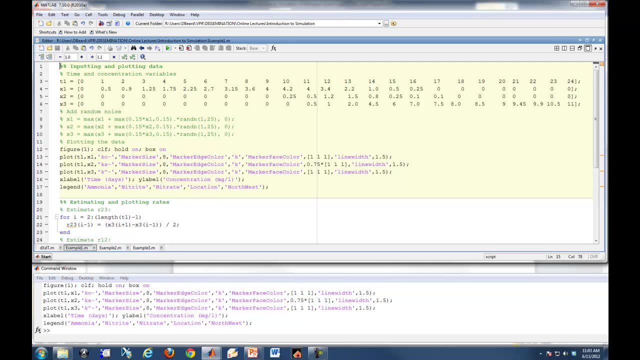 mass conservation model directly from our measured data, And how we do that is going to be illustrated by this simple example in MATLAB. So in this MATLAB code, what I have done is first of all simply input the measured data. So these data were measured by me in an aquarium in my house. 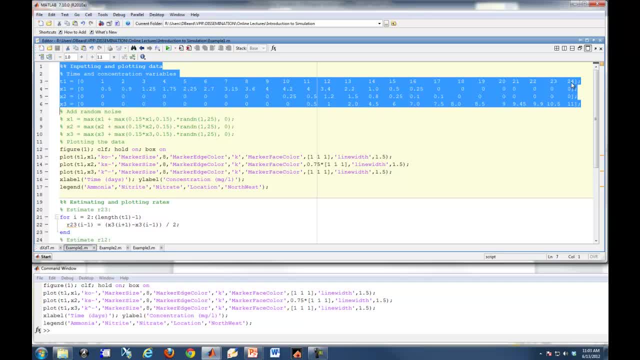 at every day for a period of a little more than three weeks. So our time vector t1, goes from 0 to 24 in steps of 1, and then we have measurements of x1,, x2, and x3,. 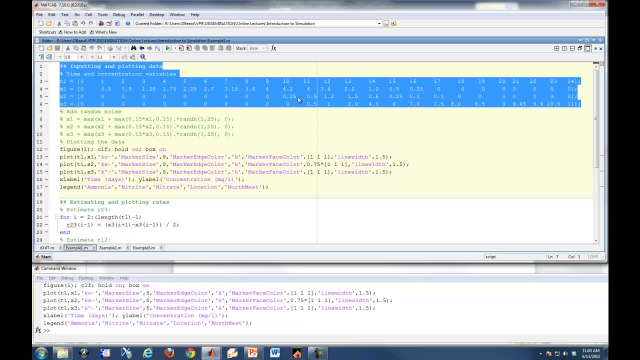 ammonia nitrite and nitrate at each of these time points. So these are our raw data and then this little piece of code here. first of all, we have some part of the. we have a random noise term which we're going to use later. 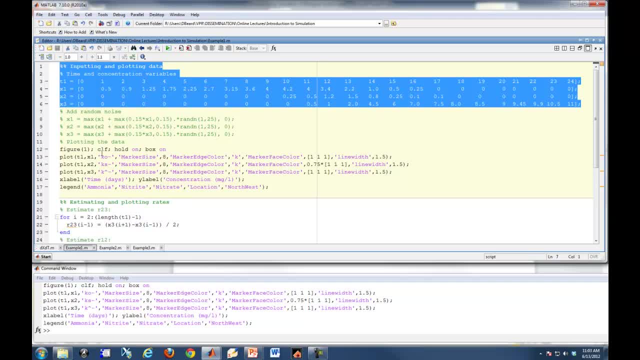 for now it's commented out. and then what this little piece of code does is it just makes a figure and it plots x1 versus time, x2 versus time, x3 versus time, and it labels the axes- x-axis- with time. 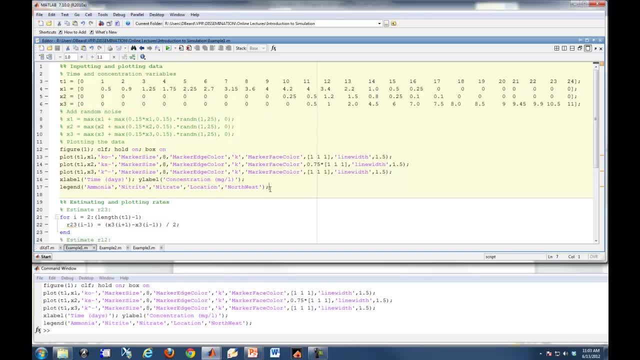 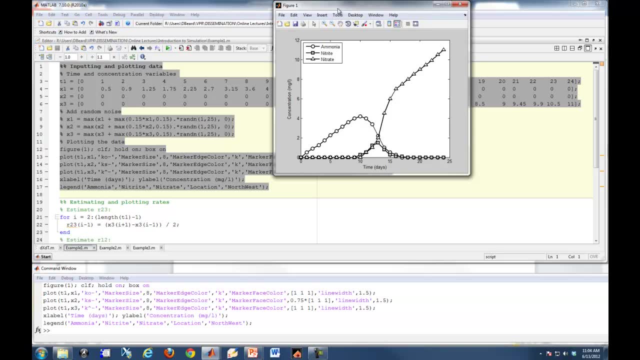 and the y-axis with concentration, and then it puts a little legend in there. So if I execute this little piece of code, we get this little figure here. Okay, That's nice. Now, looking at the rest of this code, what I'm doing is: 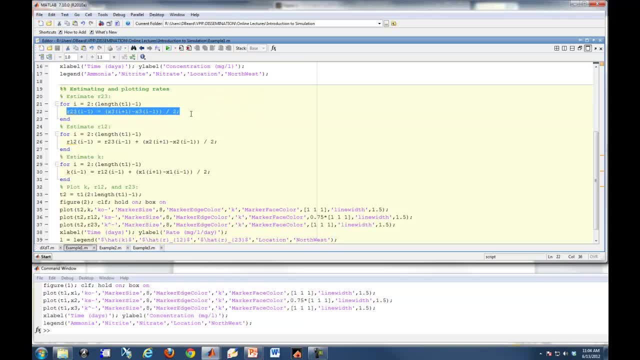 I am simply assigning those finite difference approximations. I'm looping over an index from 2, all the way up to 1 minus the length of the time vector, and that's because we're doing this centered difference approximation which we can't evaluate at time. 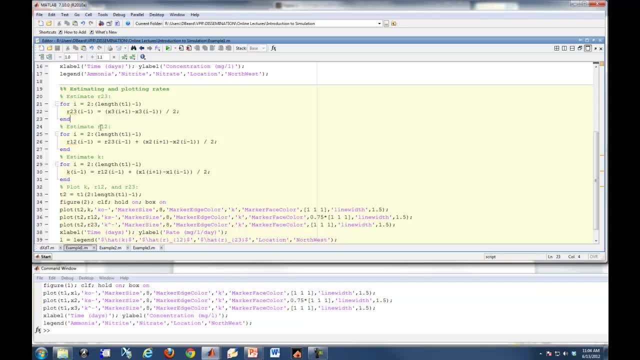 at the first time and at the very last time in the time vector, And here's my estimate for R23,. from the mathematics, we just saw Our estimate of R12, which is R23 plus the finite difference approximation for x2,. 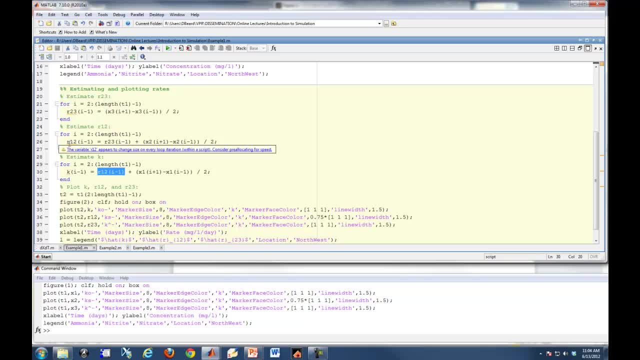 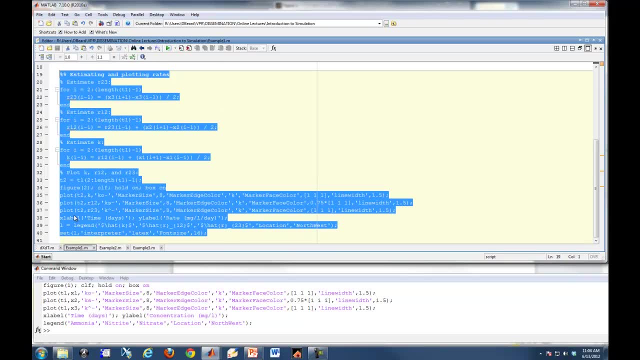 and our estimate for k is the finite difference approximation for R12, plus dx1 dt. And then what I'm doing in this little piece of code down here is just plotting the estimated k versus time, the estimated R12 versus time. 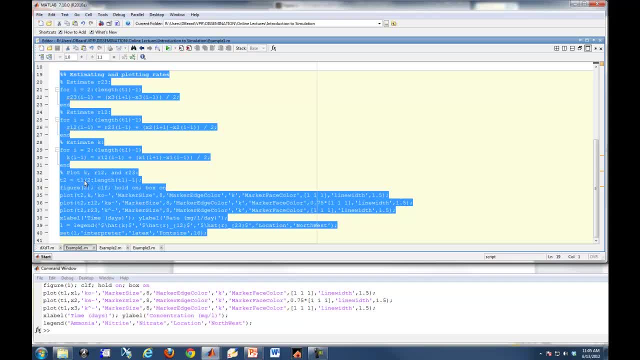 and the estimated R23 versus time. So our time vector t2, is is our time, is our original time vector. but what I've done is I've removed the first point and the last point because we don't have estimates for those rates at those points. 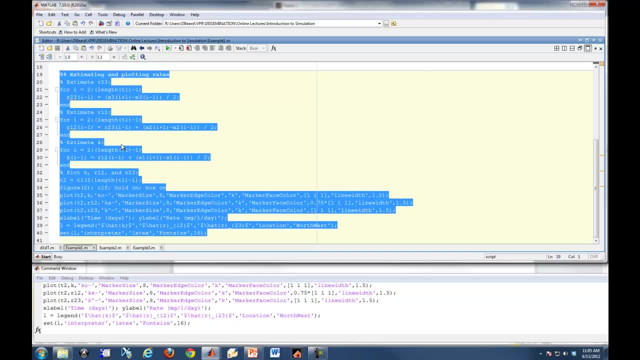 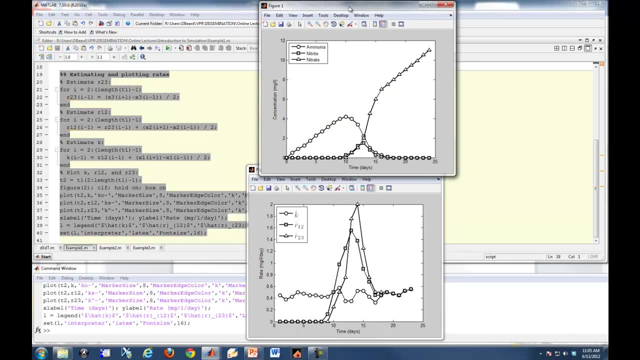 So if I execute this little piece of code here, we get a- let me find that original figure. we get our estimates for those rates, k R12, and R23. And again, there's no, there's no. 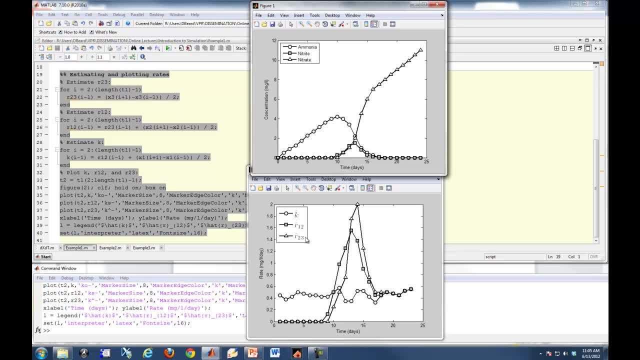 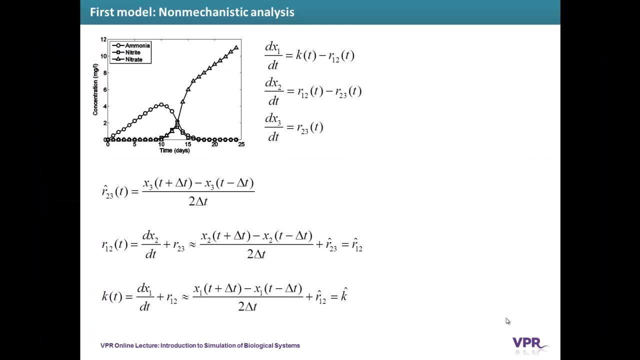 um underlying model for the mechanisms behind these uh transition rates. We've just estimated them directly from finite difference approximations of the of the um slopes of the raw data. So, going back to our PowerPoint, this is what we just looked at. 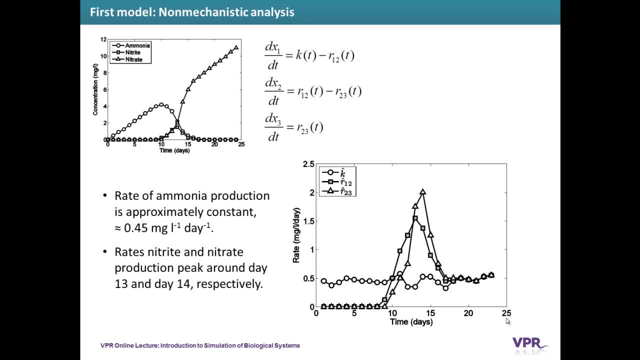 So what can we learn from that kind of analysis? Well, we can, uh, maybe glean from looking at these estimated rates that the rate of ammonia production compared to the other rates is fairly constant over the time course of the experiment. And if 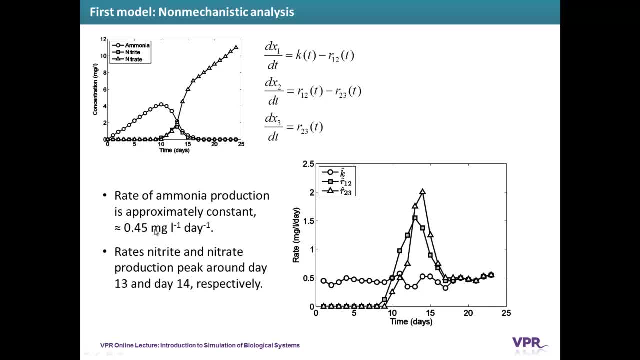 uh. specifically, it's approximately 0.45, uh milligrams per liter per day. We can also uh determine that the rates of nitrite and nitrate production peak somewhere around the middle of the experiment. Um, nitrite production peaks about a day or two earlier than nitrate production. 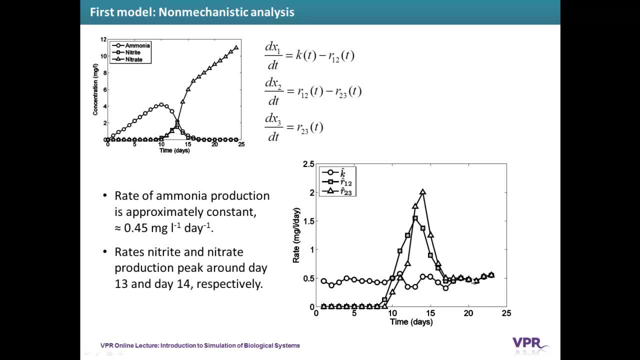 And then they everything kind of levels off in a steady state All the fluxes are are approximately the same. So the finding that ammonia production is constant is, um, I think, a result of the controlled experiment where we tried to input on a daily basis. 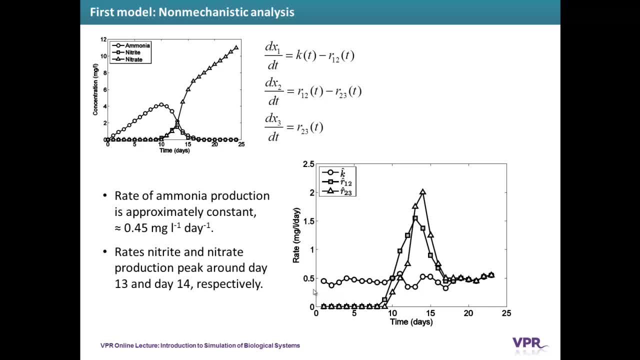 the same amount of food and therefore the same amount of protein and the same amount of nitrogen, into the system Um, and the changes in these other rates, nitrate and nitrite production, have to do with changes in the uh. 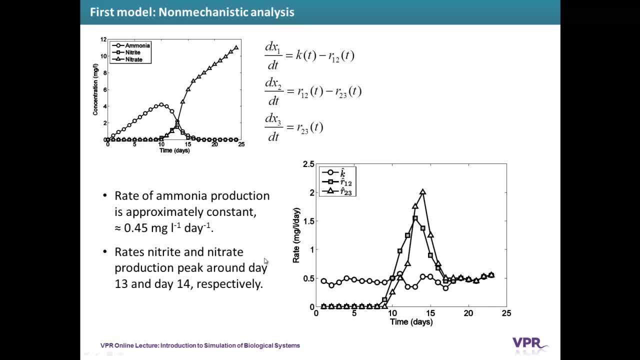 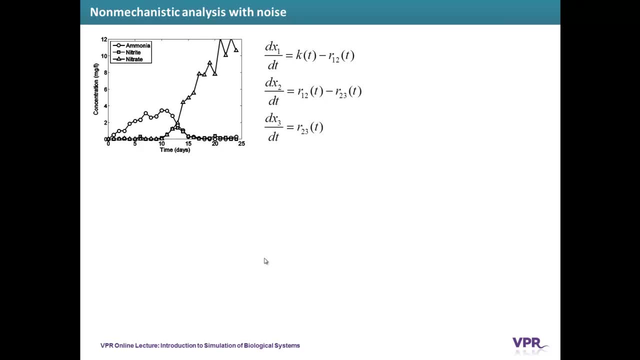 bacterial populations in the aquarium filter. So that's an interesting finding. Um again from a non-mechanistic analysis of the system. Next example we're gonna we're. what I've done here is I've added random noise to the system. 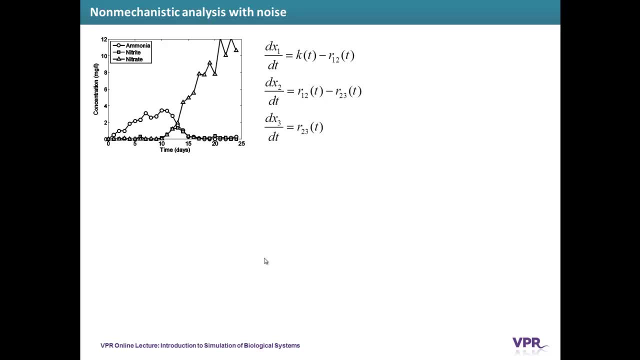 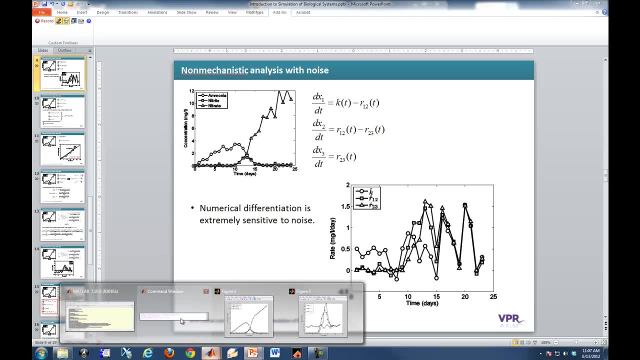 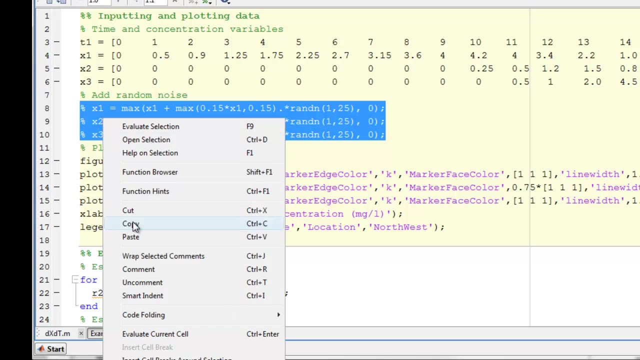 Okay and um, this is. noise is, of course, a uh, very common in biological processes and in measurements of of biological processes, And so we can explore what noise does to a system by going back to our code and um. 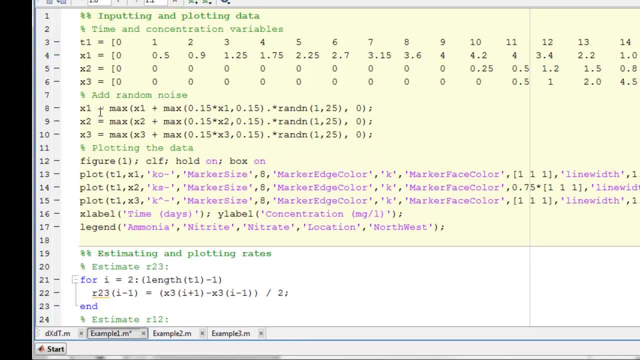 adding some random noise. So I'm I'm. what I'm doing is I'm adding noise of about uh 15% of this of the um, uh. strength of the signal for X1,, X2, and X3. 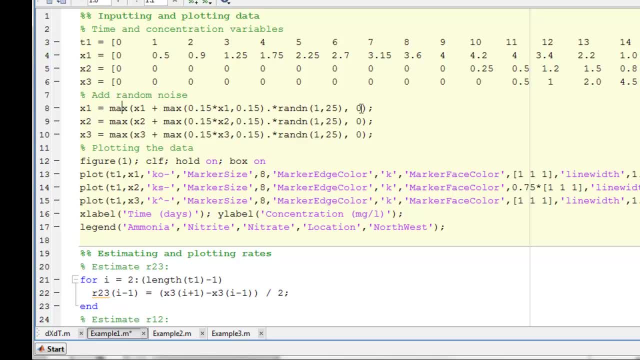 And what this max comma zero does is that it, it, um, uh, make sure that I don't get negative values of concentrations, which would be physically impossible, Um and um. what this does is it puts an upper limit on. 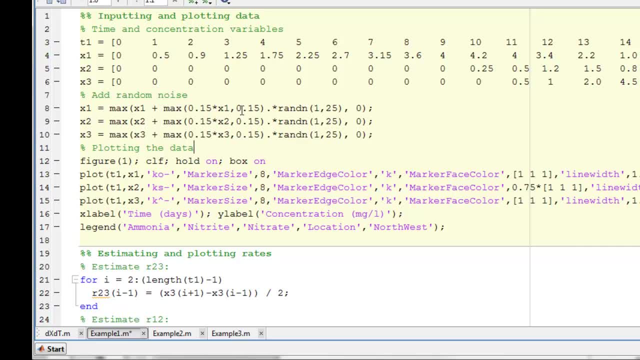 on the uh weighting on the noise of about the value of uh, um 25. on the on the noise Um, and then this just is a random vector of length 25, which is the length of the time vector of Gaussian random noise. 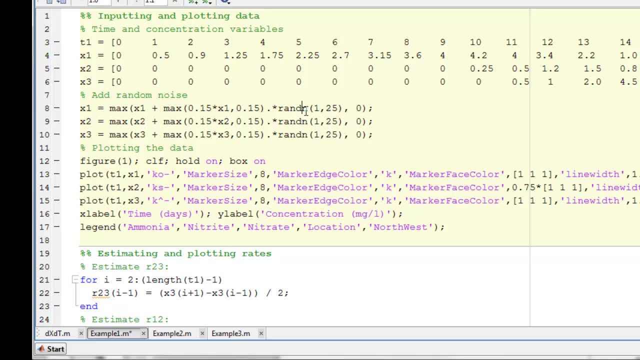 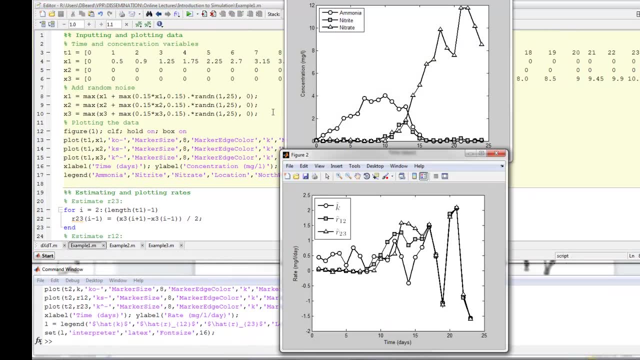 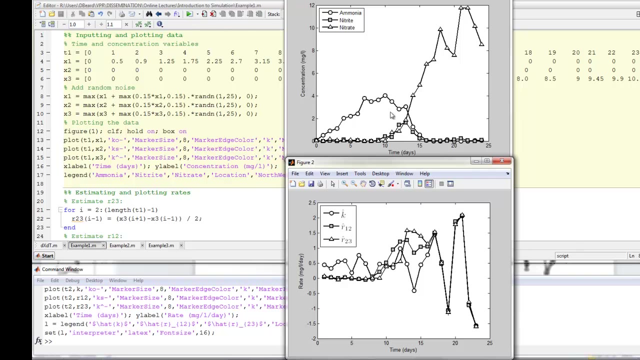 um with mean zero and uh, uh variance one. So here I can run these two codes again with noise, And here you see some noisy data. It's not exactly the same uh data set that you saw on the slide, because every time you run it. 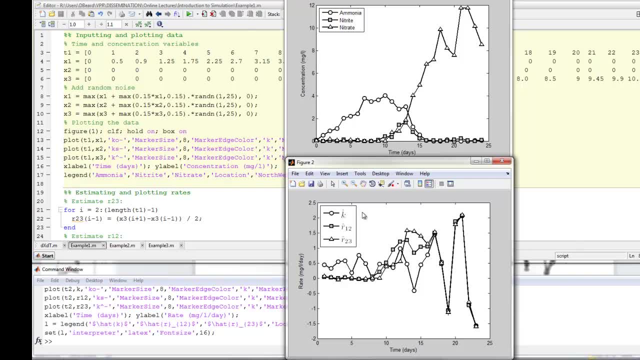 it's a different realization of randomness And, uh, when we apply our finite difference approximations, we get something that really doesn't look very useful or very good here for our, our fluxes. Okay, And you know if we want to. 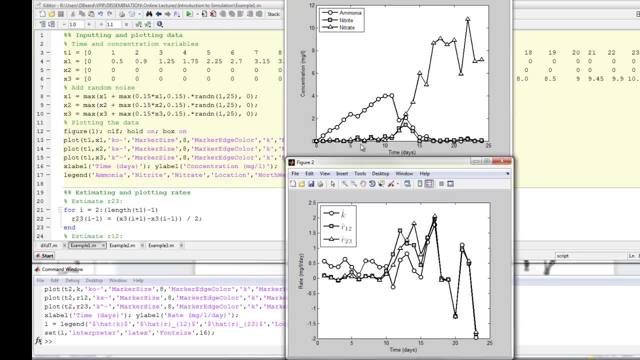 we can run that again. We get something different, but still something that looks terribly messy and terribly noisy. Um, where you can see the amount of noise in in the system here. um, uh, where you know the the basic trends are. 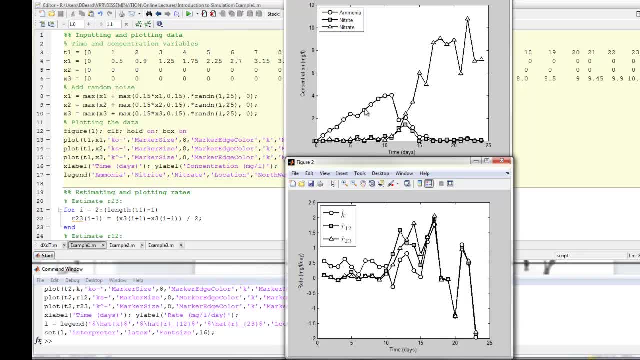 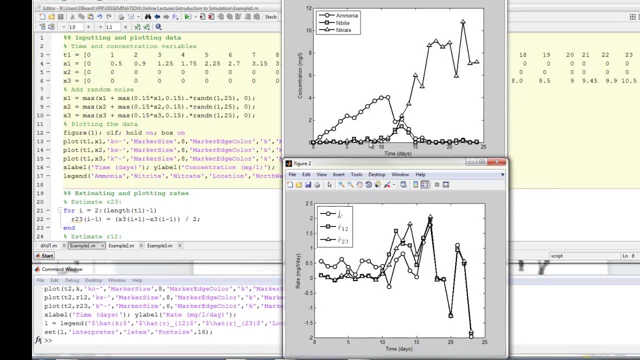 are still apparent: Uh, buildup of ammonia, and then, um, um, followed by this, this decrease buildup of nitrate, followed by this decrease in this kind of steady buildup of of nitrate. So, briefly going back to our PowerPoint, 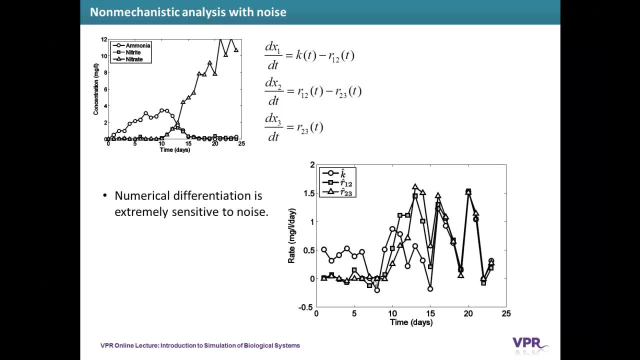 um. there you have it. So this is for this particular realization of the noise. this is what the numerical differentiation gives us, And the lesson here is that numerical differentiation is extremely sensitive to noise. Um, uh, in. in very basic terms, 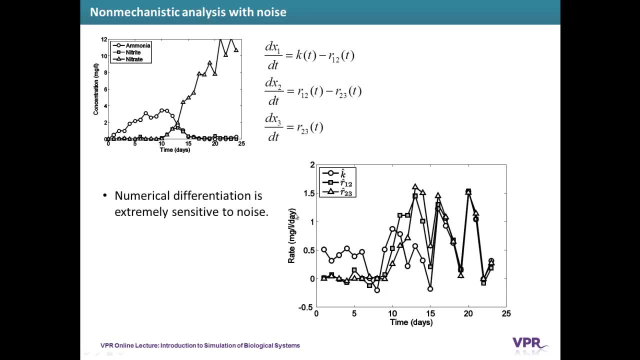 And this analysis doesn't work very well and doesn't provide very much useful information when we have noise on a level of of, say, 10 or 15 percent, which is what we're dealing with in this example. So so what can we do? 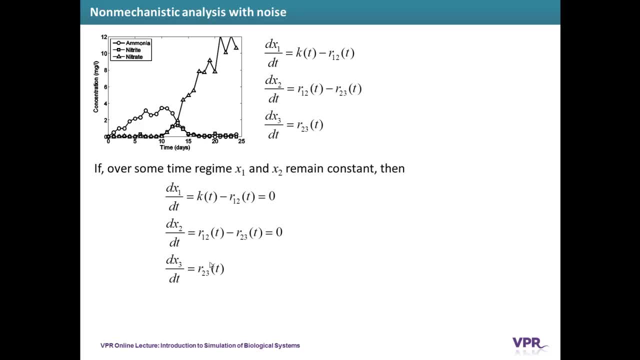 Well, we can um go back to our data and go back to our raw equations And, for example, one thing we might notice is that you know, after about the second, uh, um, you know, these rates of change of x1 and x2,. 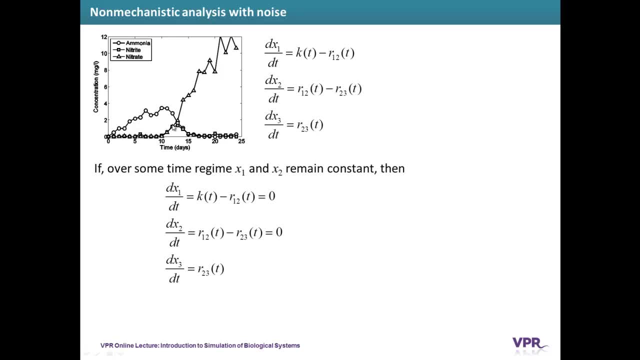 uh, uh go to zero, at least compared to these rates of change early in the experiment, compared to the rate of change of x3.. So these values are not only approximately zero, but they're um, they're not changing. 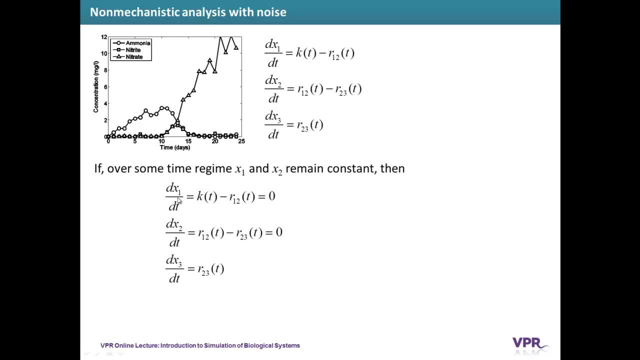 So over some time regime maybe we can notice we can approximate these derivatives as zero And if we do that we find that r1, 2, is equal to r2, 3.. Okay, and if r1, 2 is equal to r2,? 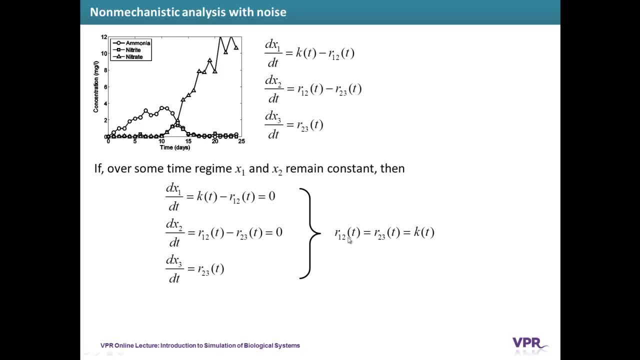 3, then it's also equal to k, right? And so all of these rates become equal at some sort of um when x1 and x2 reach some kind of steady state. Well, that's interesting. How can we estimate that constant rate k? 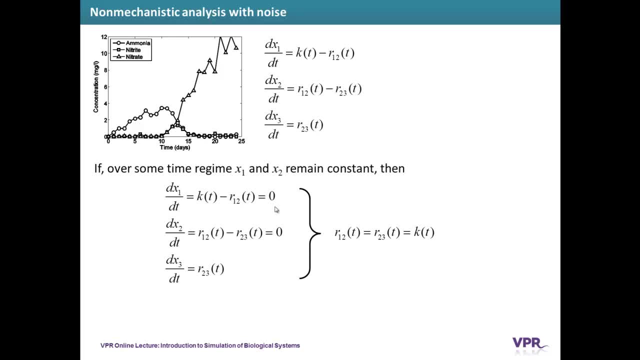 And what could we learn if we are able to estimate that constant rate k? Well, another thing we can do, um is just add up these equations And we get the and. and what happens? when we add up these equations, we can notice that this term and this term cancel. 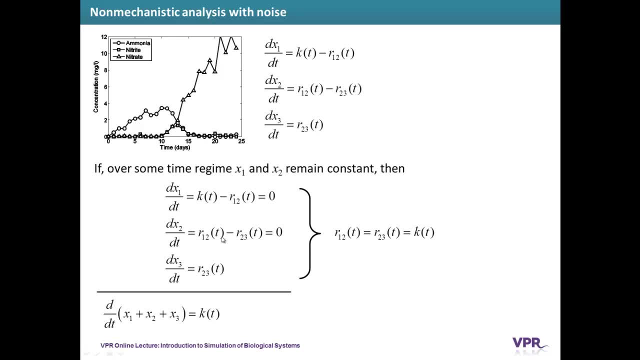 this term and this term cancel, and the rate of change of total nitrogen in the system- x1 plus x2 plus x3, is the rate of input of ammonia into the system, because it's the only source of nitrogen that's being input in. 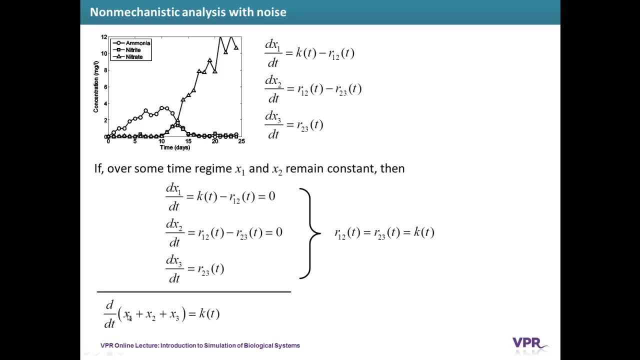 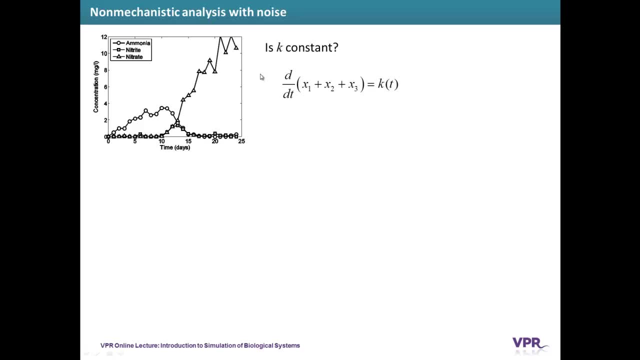 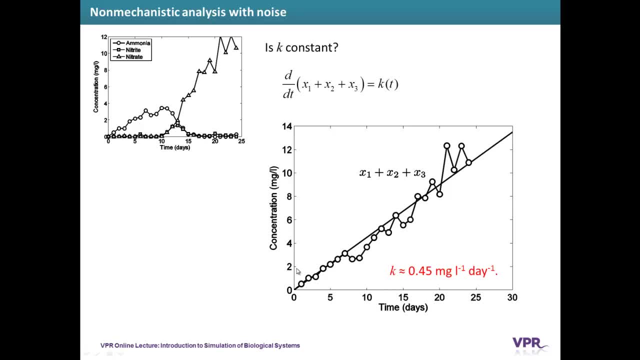 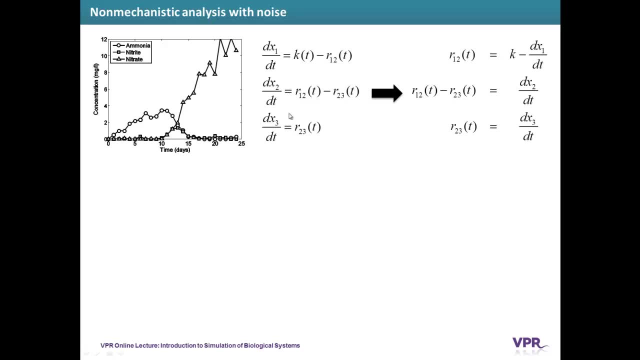 very simple. We take our set of equations and we write it in a more convenient form where our unknowns, our r12 and our r23 on the left hand side, and what we're going to put on the right hand side are things that we know and are things that we can estimate. 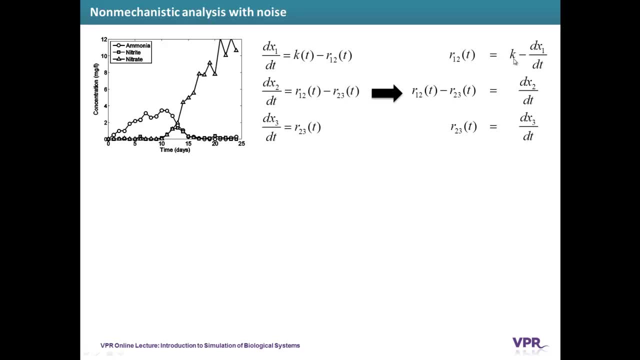 So we have an independent estimate for k from this analysis here And we're going to assume that we can estimate dx1 dt, dx2, dx3 dt this way. It follows from our finite difference approximations. So now we have three equations and two unknowns. So that's a mathematically 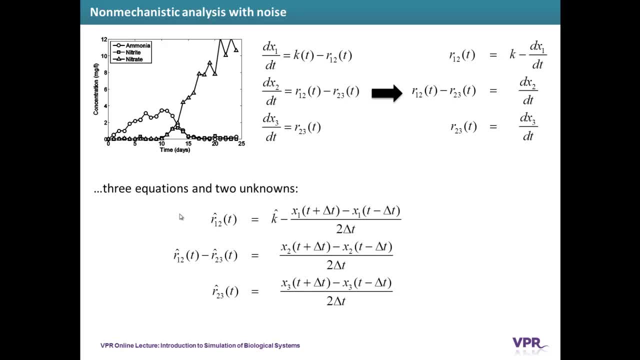 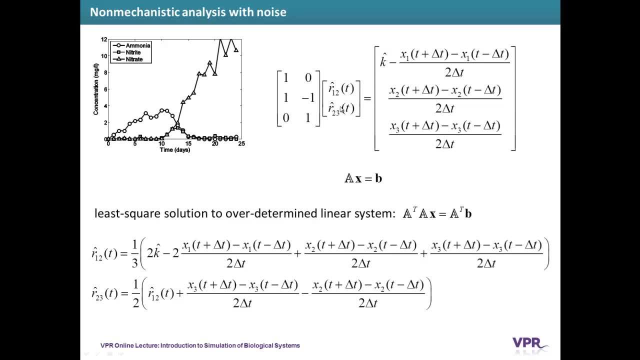 underdetermined problem. Three equations are two unknowns. The two unknowns are r12 and r23.. What can we do with that? Well, I'm just recasting those same equations in a slightly different form, some sort of a matrix, vector form, where 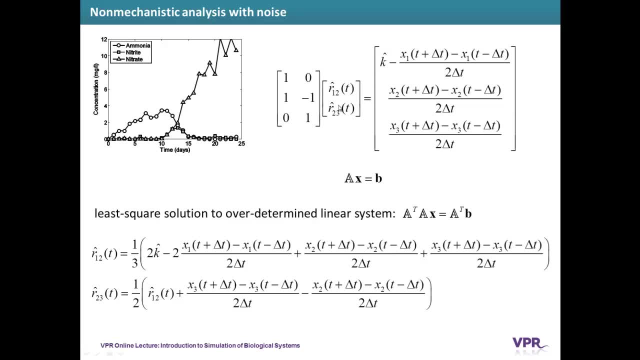 a is a matrix of these coefficients. x is our vector of unknowns here- r12 and r23, and b is our data on the right hand side. Okay, so there's a general solution to this kind of loop. This is a linear least squares problem, Okay, and that is given by the following mathematical: 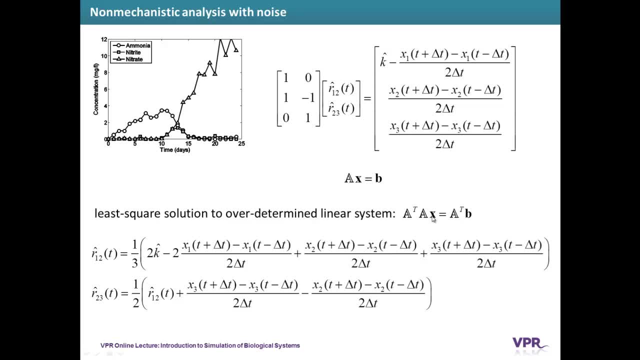 solution to the following mathematical expression. We take a transpose times a. x is equal to a transpose times b. This is a well-posed system And you can look up the details to how we can translate this equation into this equation in order to get the least squares. 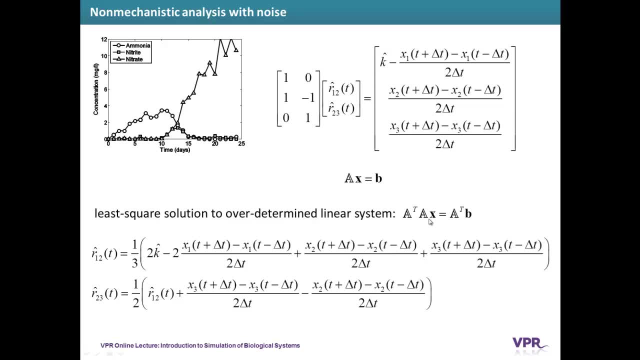 solution to a: x equals b. Okay, put that, let me say that a different way. The solution to this equation is a solution where the sum of squared differences between a, x and b is minimized. Okay, and doing the algebra which I'm not going to show you here, the 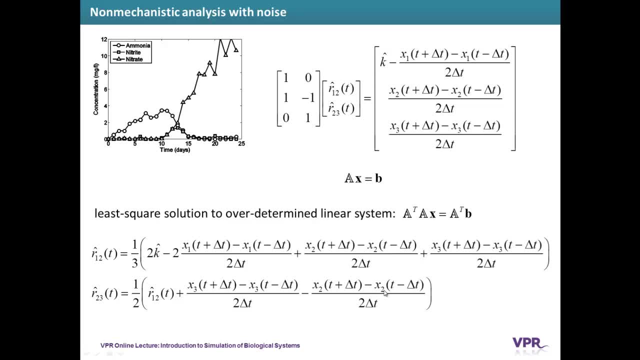 solution to this equation is given by this kind of long, complicated things, But it's simply some kind of linear combination of our estimated k and our linear least squares and our numerically estimated derivatives for r12 and r23.. So what can we do with? 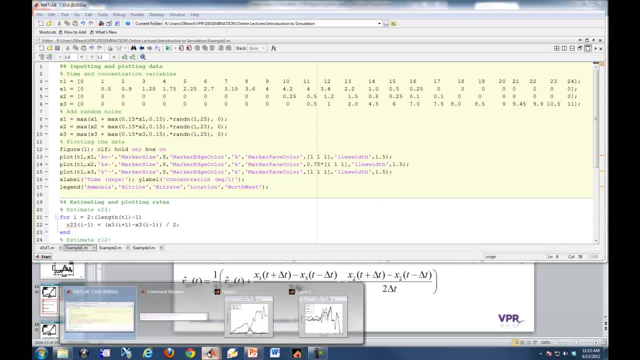 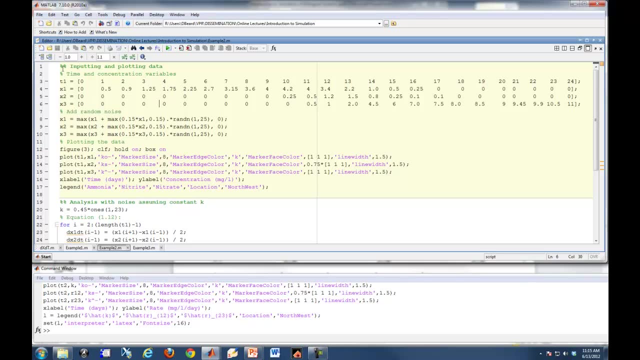 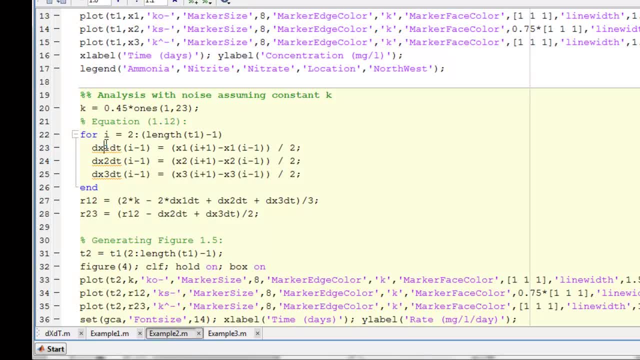 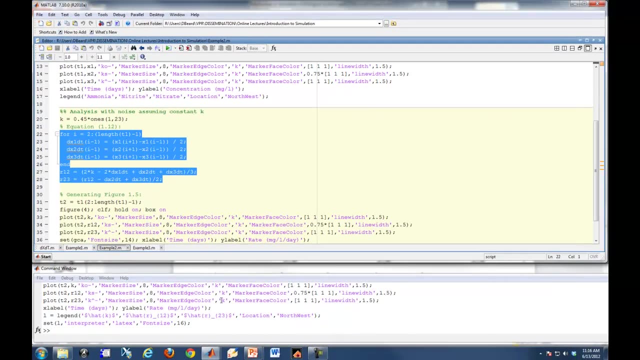 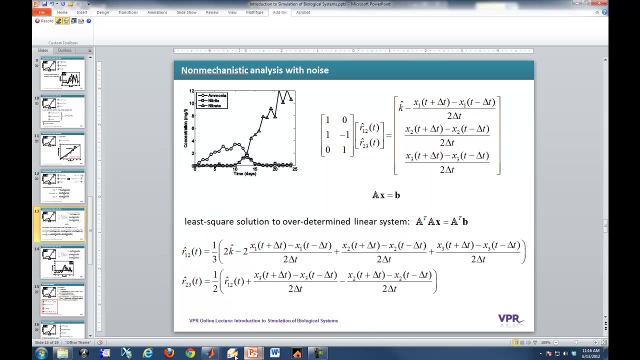 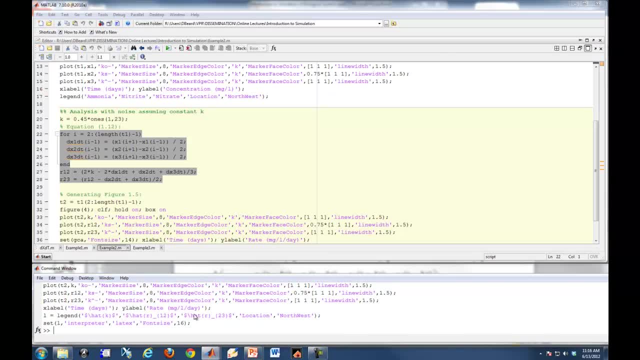 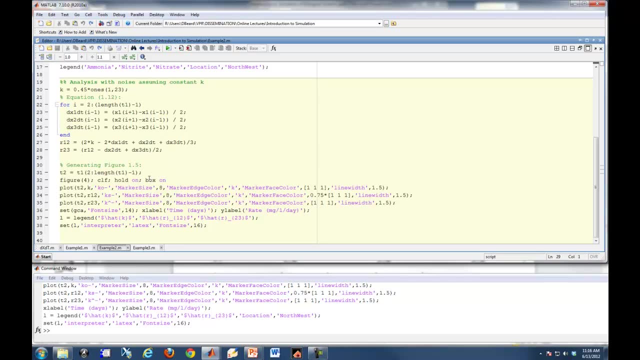 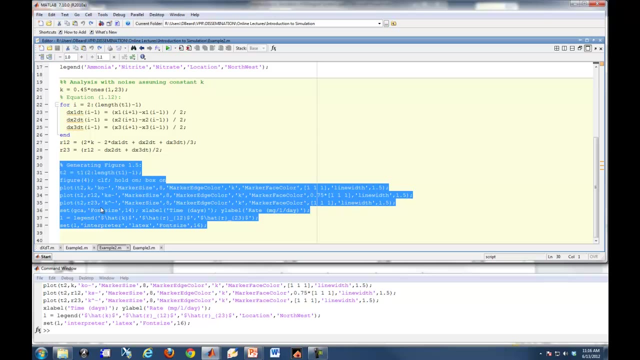 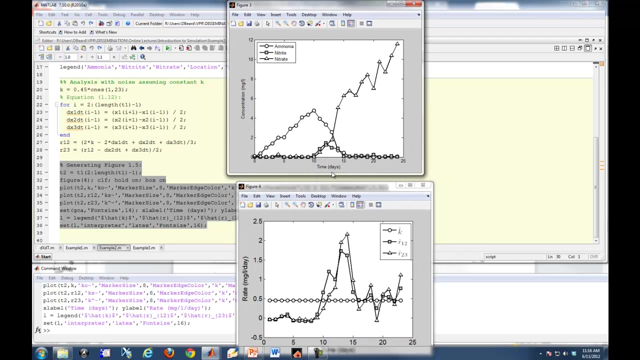 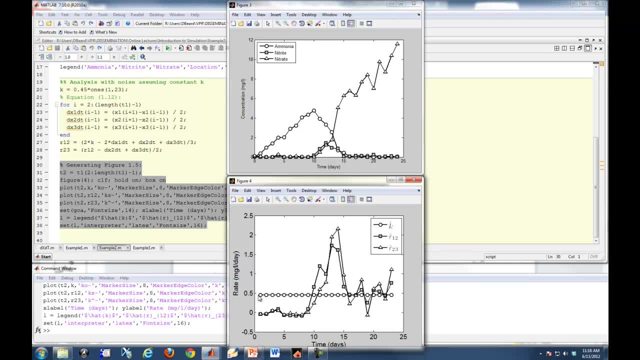 and for the k and those rates. and of course, as i said, we've made an input assumption into this analysis that k is constant, so this is the constant k, and then we see something that looks a little cleaner, a little better than our previous analysis, where we actually see 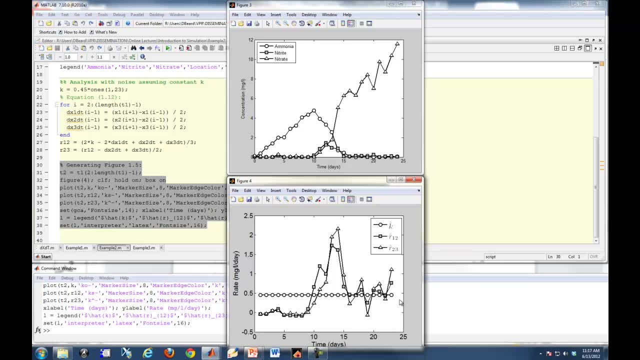 that these peaks occur for r1- 2 and r2 3. uh, and it looks uh a lot more like the information we can get from our noise free analysis, okay, and just uh, uh, showing that everytime we run this we're going to get an. 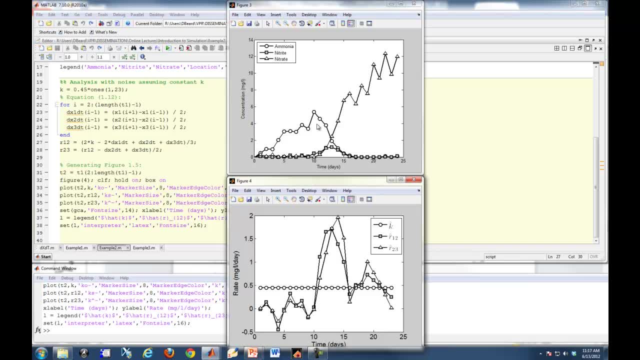 assessment slightly different behavior because it's a different realization of the noise. The trends are the same. We still see this kind of behavior which we think is not realistic. That is, some of these rates are going negative. We don't expect to see that Physically. we don't expect to see 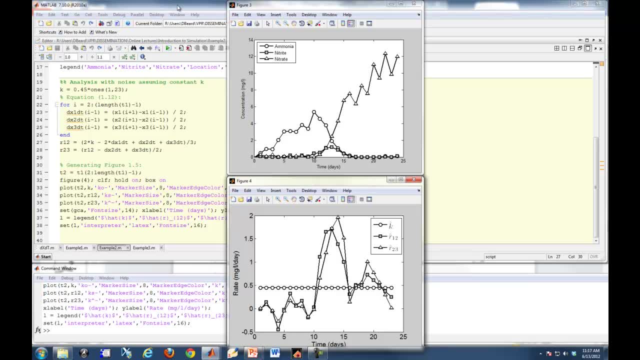 these oxidation reactions going in reverse. But maybe we don't know that in pre-order, I don't know. There's another realization. This one looks a little worse because we have some apparent negative fluxes that are of the same order of magnitude as our positive fluxes. 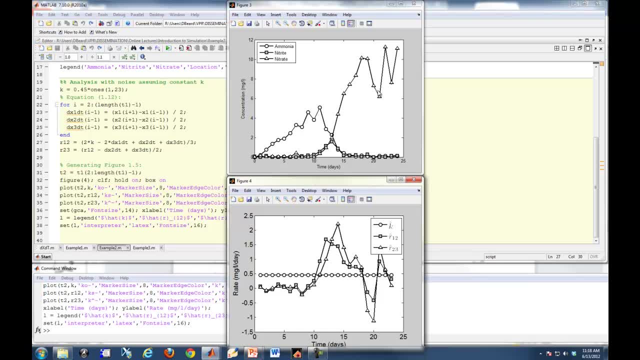 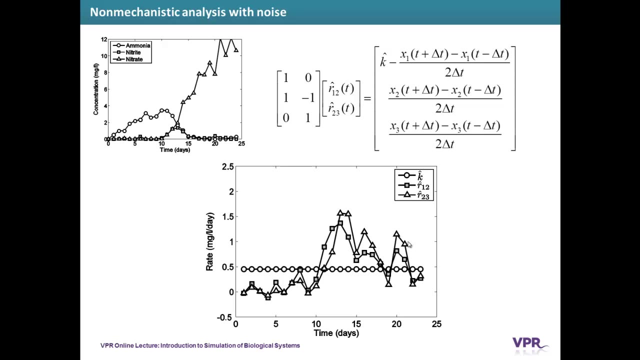 That apparently has to do with these big, strange swings in the data here. Just one more time for fun. That one looks a lot better. So back to our PowerPoint. Here's a realization of that analysis based on this particular noisy data set which is illustrated here. So again we see. 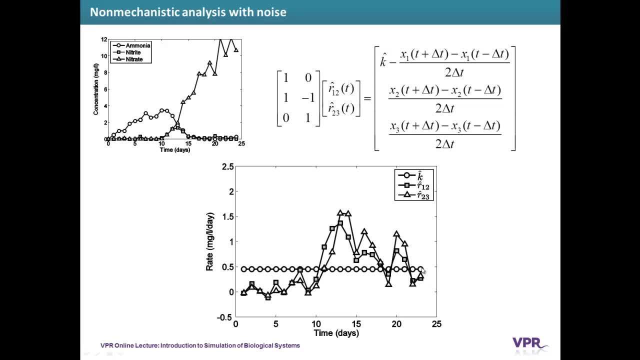 the constant rate which we input, Constant rate of ammonia production k, And we see that the oxidation by the nitrifying bacteria don't tend to be turned on until somewhere around the middle of the experiment, where they peak and then they decay down a little bit, But again we see some funny oscillations. 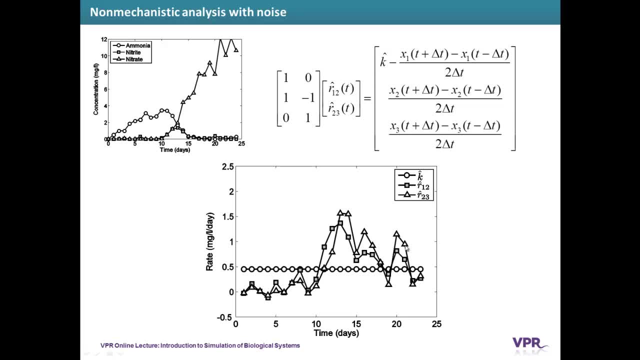 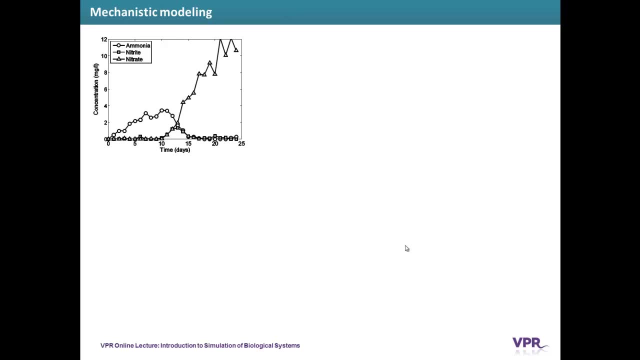 which are due to the noise in the system. So that's what you can do With a quote-unquote, non-mechanistic analysis. Next thing I want to talk about is what I refer to as mechanistic modeling, That is, can we build a model of the system in order to simulate the processes? 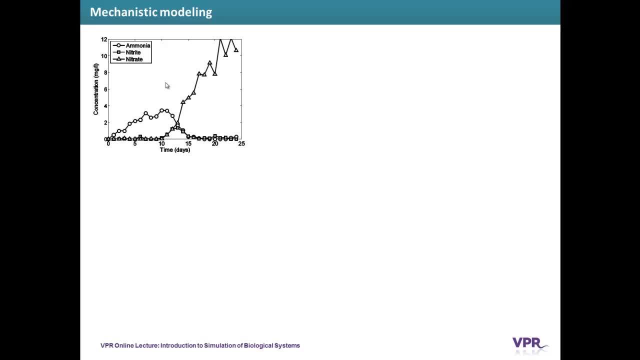 that are going on. The way we do that in general is we start with making a list of assumptions and then translating those assumptions into mathematics, And this is a process of mathematical modeling. So, for example, we could invoke the assumption that k is constant. 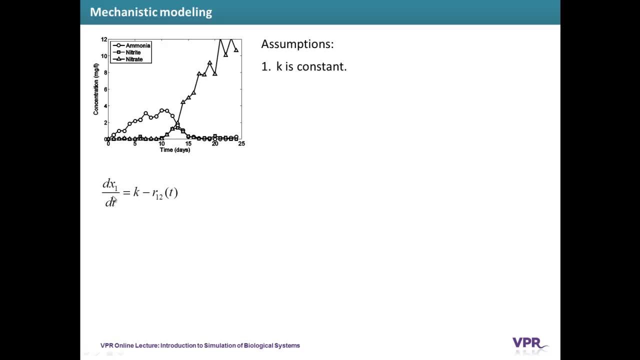 So if we evoke that assumption, we have our equation for x1, dx1, dt, which is the same equation we had before, except formally. I'm not putting k here as a function of time, So I'm saying k is a constant If we want to. 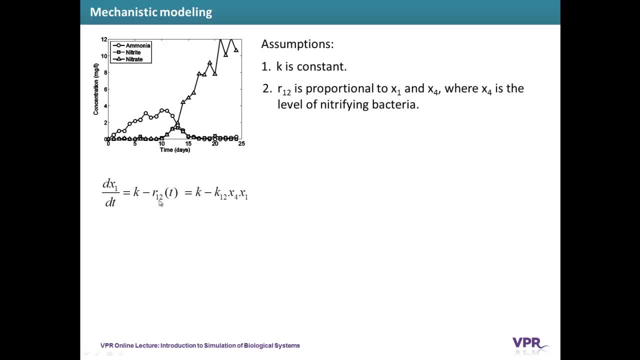 invent an expression to try to model R sub 1- 2, we might assume that, or at least guess that maybe R sub 1- 2, that rate of conversion of x1 to x2 is proportional to x1.. x1 is a substrate for that reaction. 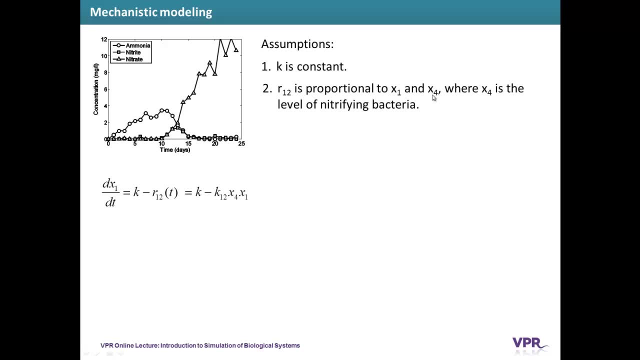 And it might also be proportional to x4, which is a new variable I haven't told you about yet. We're going to put it in the model. x4 is the level of nitrifying bacteria in the system, So x4 is going to change with time. 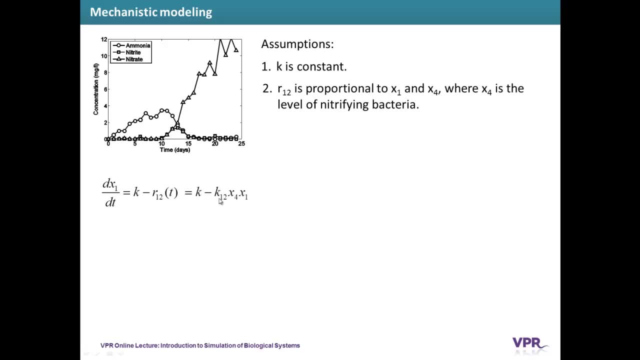 So, putting this assumption into mathematics, we have some constant k sub 1, 2 times x4 times x1 for this equation here. Okay, next equation R sub 2, 3, that's, this term is proportional to x2.. 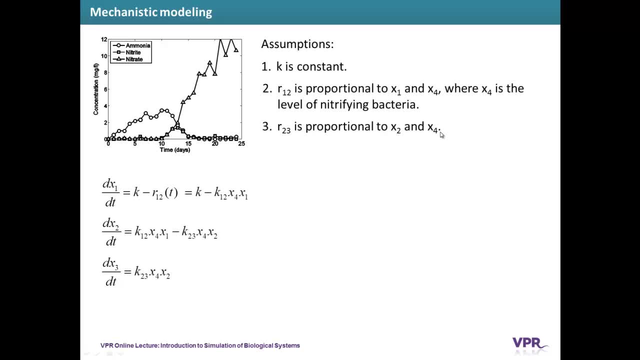 That's the substrate or the food for that reaction. It's also proportional to x4. So we have one population of nitrifying bacteria, which may be a good enough assumption, or it may be an oversimplification. We'll see when we 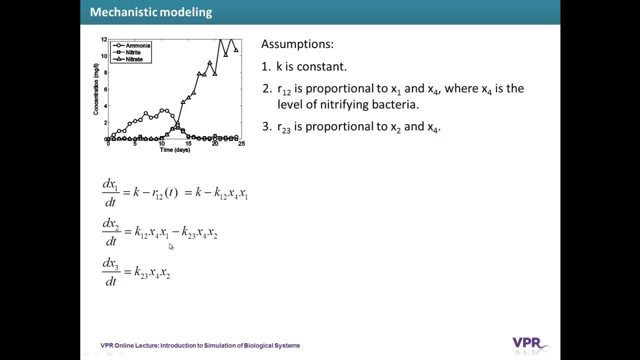 analyze and simulate this model. So R sub 2, 3 comes here with a negative in our x2 equation and it comes here as a positive in our rate of production of nitrate. here, Finally, we need an equation for x4, the growth of bacteria. 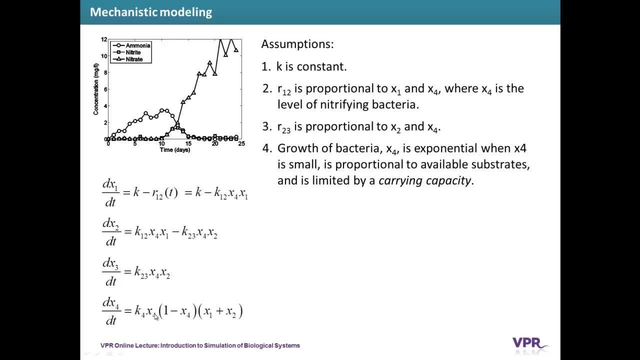 So the assumption here is that x4 grows exponentially when x4 is small. So when x4 is small, this term is essentially 1. And the rate of growth of bacteria is proportional to the population itself. That's exponential growth. We also say it's proportional. 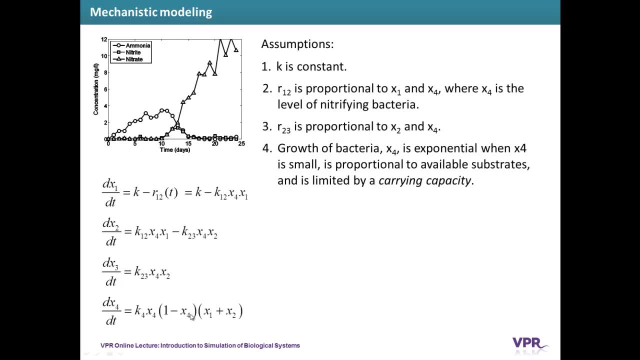 to the food that those bacteria are eating. And since we're assuming one common pool of bacteria which is responsible for both oxidation processes, the total food available is x1 plus x2.. Okay, So we're treating x4 as an element of oh. and then finally, 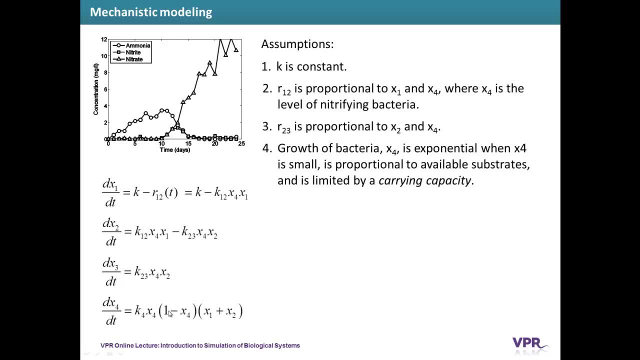 growth is ultimately limited by some carrying capacity. So we're treating x4 as a non-dimensional population level here, where one is the carrying capacity And so when the growth, when they've gone to the heck своей green, so the amount of bacteria. 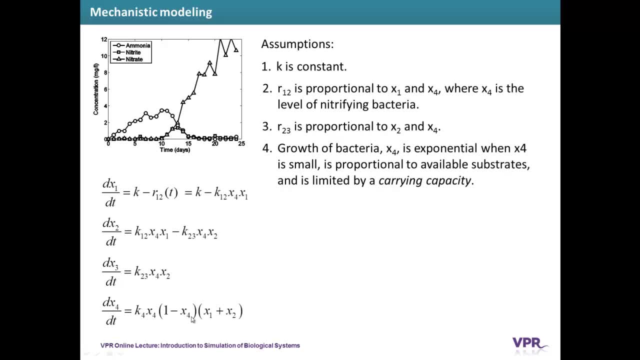 X4 approaches 1, then it can't grow anymore. So this equation is an ecological model commonly invoked It's called the logistic growth model. You can look up more details on that. We'll just see how it behaves in our system. 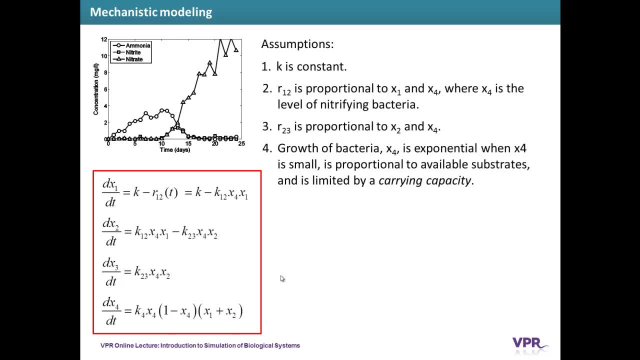 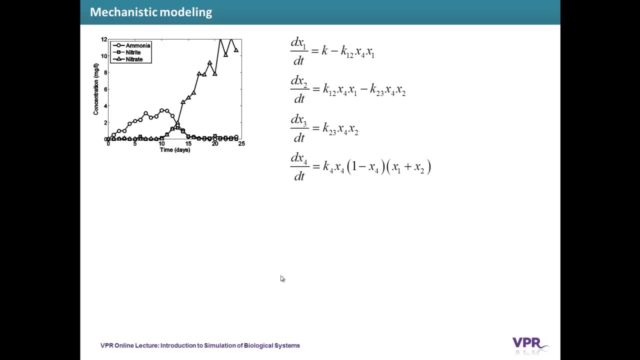 So that's our model: A set of four differential equations. These four differential equations for three measured variables plus one unmeasured variable of bacterial population. Those are those equations. again, I'll just move to the top of the page And if we want to simulate these equations, what we need 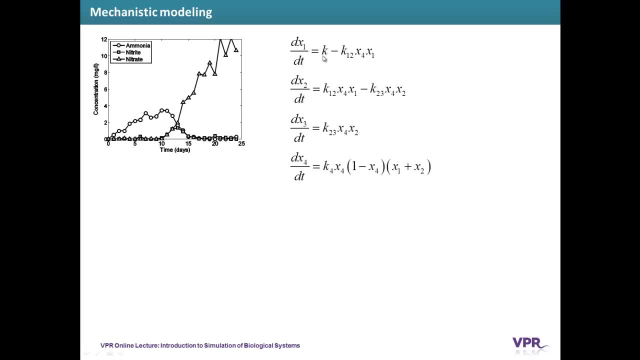 are values for the parameters. these rate constants as K1, 2, K2,, 3, K4, etc. in the model. So what are the parameter values? Well, we really don't know, And one thing we can do is we can try to take. 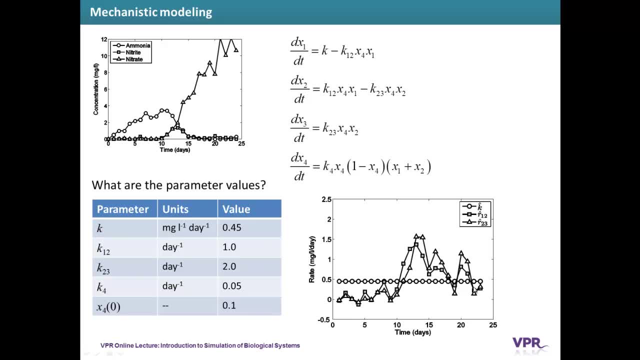 a guess. So let's look at our noisy data set and our estimates of those rates from our noisy data set. Okay, and so try to assign values to these parameters. So the first parameters, our first one, is this: constant rate K. Well, we've already estimated it to be about 0.45 in these units. 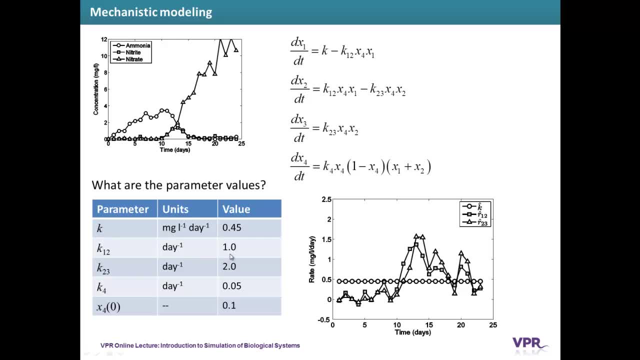 Okay. well, what's K1, 2?? Well, that's interesting. So K1, 2 tells us what the flux of ammonia to nitrite is. Okay, so we know that when ammonia is order of magnitude 2,, 3, or 4,. 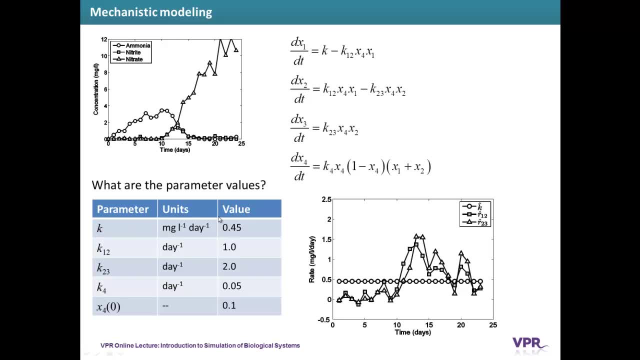 okay, the flux has to become order of magnitude 1.5. So arbitrarily we might guess as an initial guess that this K1, 2 is 1.. So that means that when the ammonia concentration is 1,, okay, the flux is K1,, 2 is about 1, assuming that the bacterial population is on the order of the carrying capacity. 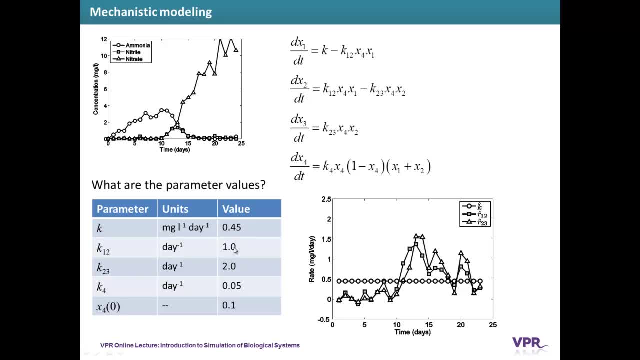 So, again, this is a pretty, very, very rough kind of way to assign these parameter values, And we're going to try to do something a little bit more after we go through this exercise. we're going to try to do something a little bit more rigorous. 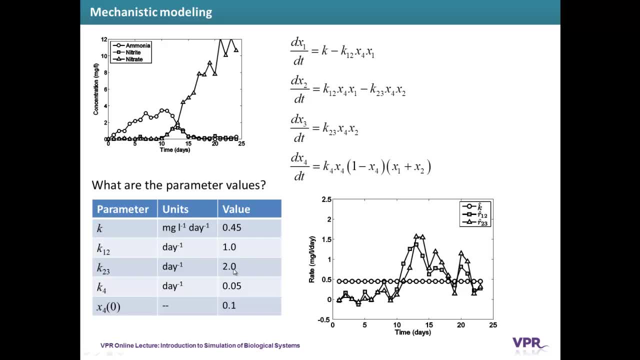 We can go through the same kind of arguments and we can make a guess for K2, 3.. And K4, which has units per day, we're going to say is about 1- 20th. Where do we get that? Well, just by looking at the timescale of the experiment. 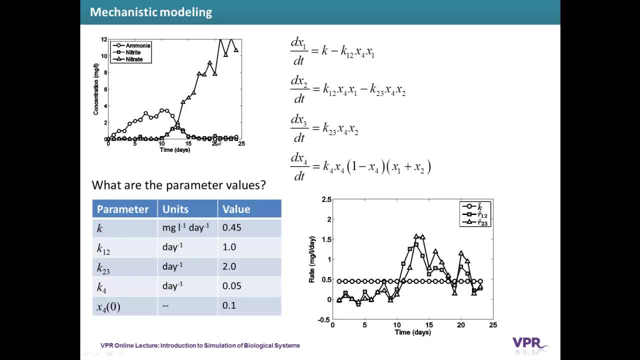 So things tend to settle down over a timescale of about 20 days. So we'll say that it takes 20 days for the you know is our, is our, you know, exponential time, growth time for our bacterial population. 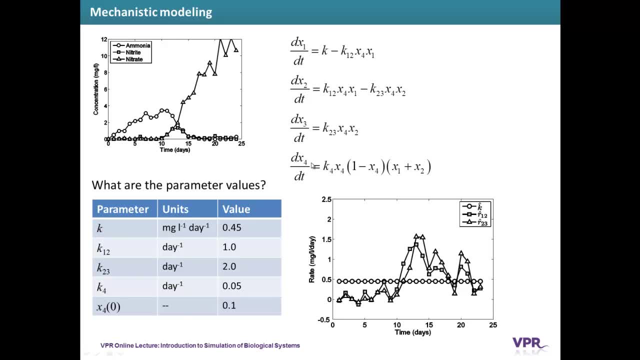 Again arbitrarily assigned, And then, since we don't have any data on X4, we actually need an initial condition. So this is the seed population of bacteria. We know that 1 is the carrying capacity, so we expect our initial condition to be something less than 1.. 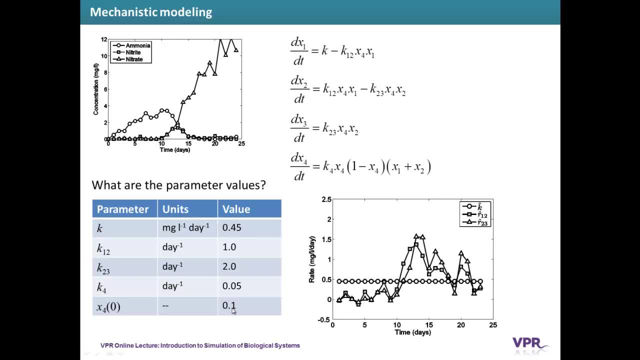 And we might arbitrarily choose 0.1. Okay, why? why 0.1?? Maybe we should. we could choose something much smaller than 0.1.. We know it's. we know that it has to be non-zero. 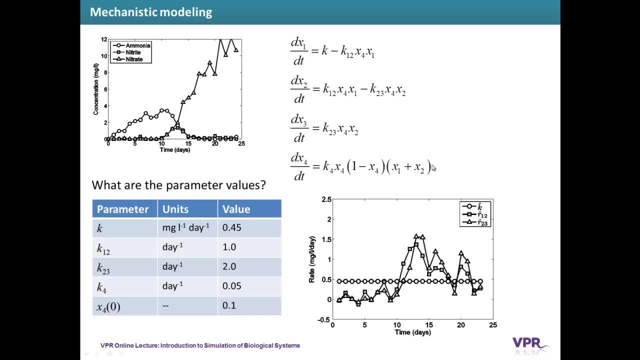 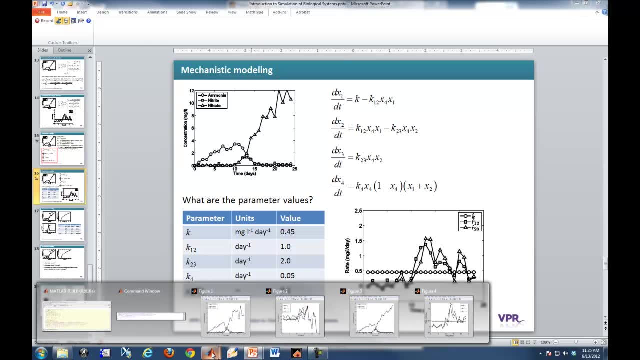 or else we'll never. if the initial condition is 0,, we'll never get any bacterial growth. We know it's something smaller than 1, so let's just try this value here. So how do we simulate this model? Well, to simulate this model in MATLAB. 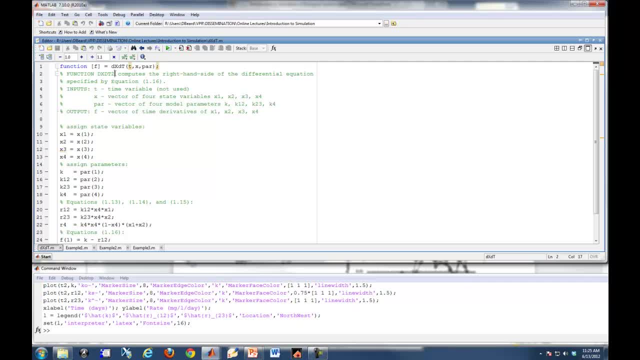 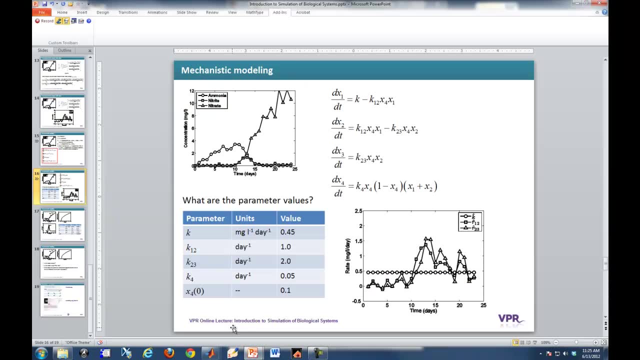 we need a function which computes the right-hand side of this set of differential equations. So go back to our PowerPoint for a minute. Here are our differential equations. The right-hand side are all of the things on the right-hand side of this dx, dt terms. 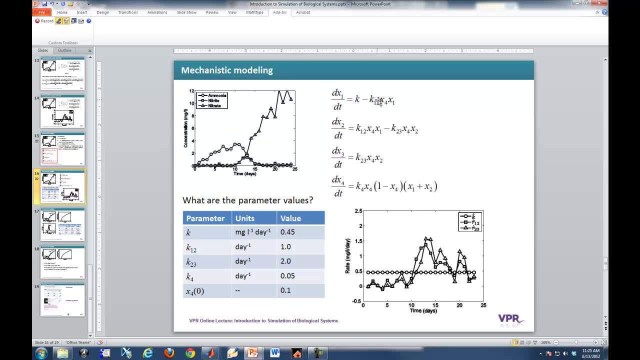 Okay, so we need to be able to compute dx1, dt, dx2, dt, dx3, dt, dx4, dt as functions of the variables, the state variables x1 through x4.. Okay, So that's what this function is. 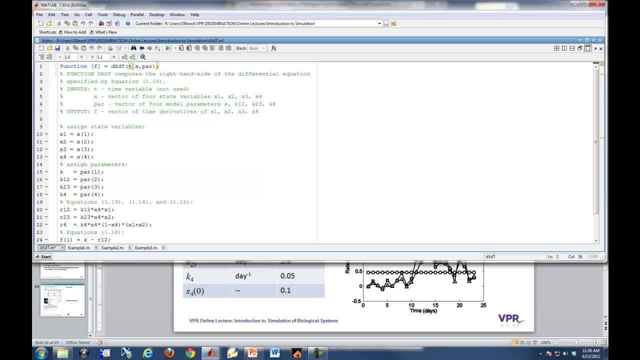 So it takes as arguments t, which is our time variable, and the ordinary differential equation integrators that I'm going to use in MATLAB require that the first argument is time. As you can see, time is actually not used in this function, but it has to be there as a placeholder. 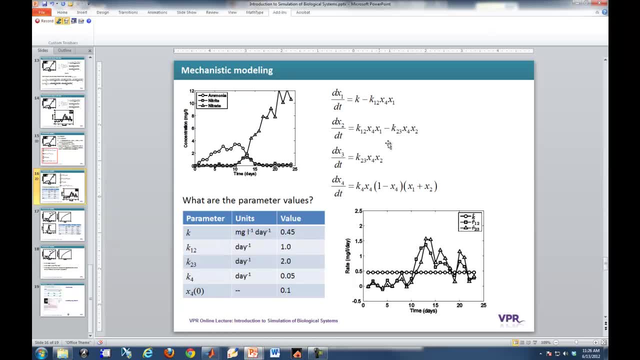 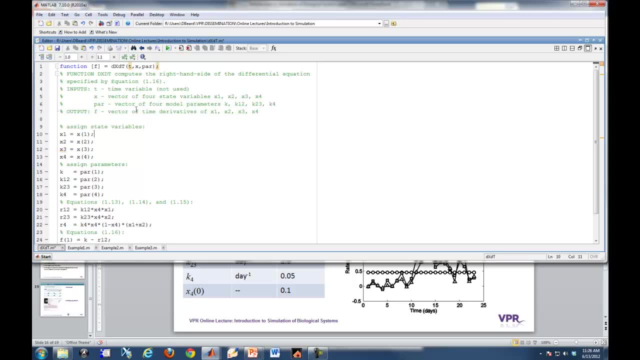 So what do I mean? it's not used, So t doesn't appear explicitly on the right-hand side of these equations. So these equations are not time-dependent in that sense. x is a vector of our four state variables, x1 to x4.. 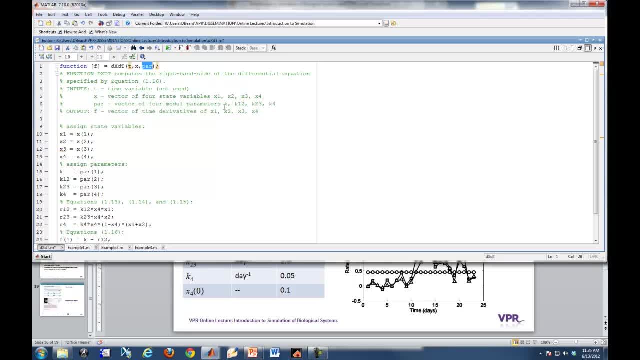 And then I've put our parameters, which are our rate constant parameters, which are k, k12,, k23, and k4, into a vector which I'll call par for parameters, And f is the output of those time vectors. So just for simple bookkeeping, 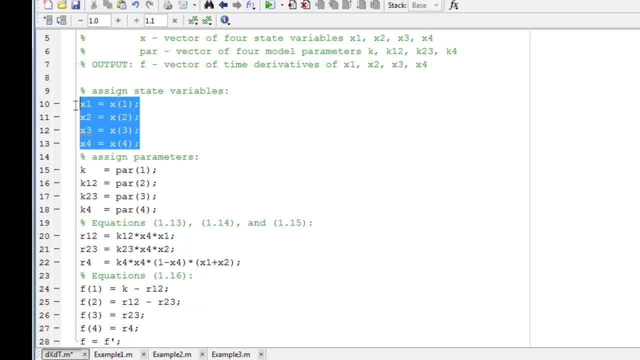 I'm going to assign x1 through x4 to the entries of x, x1 to x4.. I'm going to assign the parameters here: parameter 1,, parameter 2, parameter 3, parameter 4.. We compute our rates. 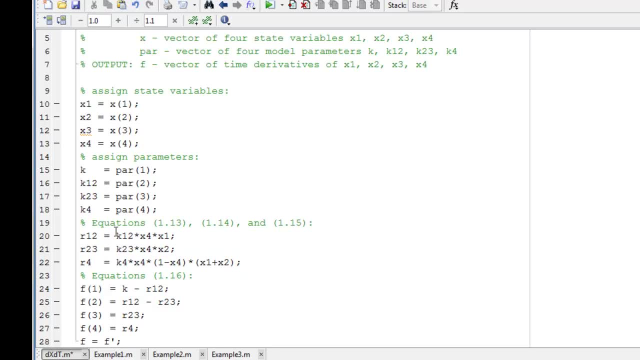 From our simple model. right, This is our mass action model for r12, our mass action model for r23, and our logistic growth model for r4.. And then these are our differential equations. Okay, now how do we do that? 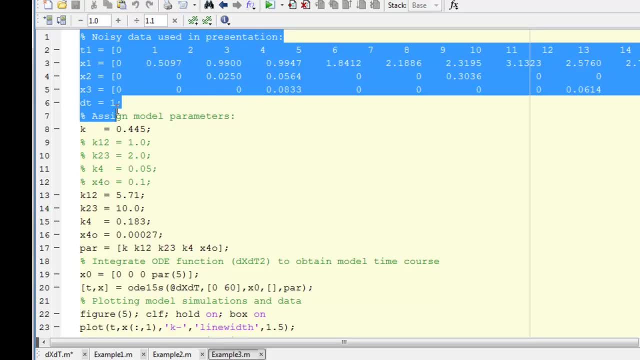 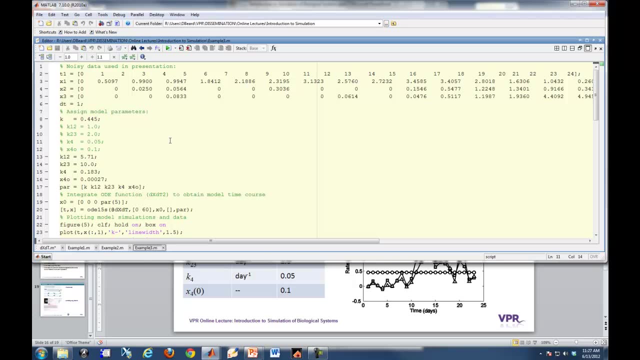 So here are our noisy data. Okay, this is not we can look at. we'll lay around, we'll look at this model simulations against our noise-free data, okay, And then, oh, let me comment this out and uncomment these. 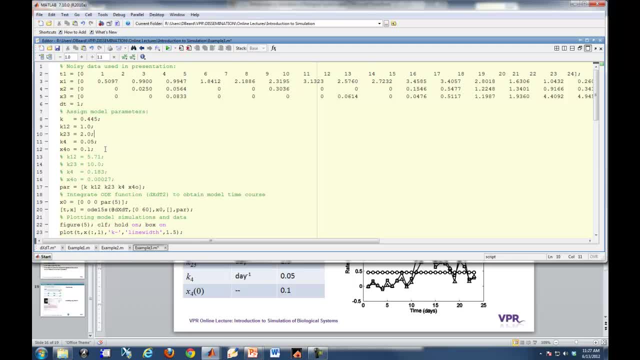 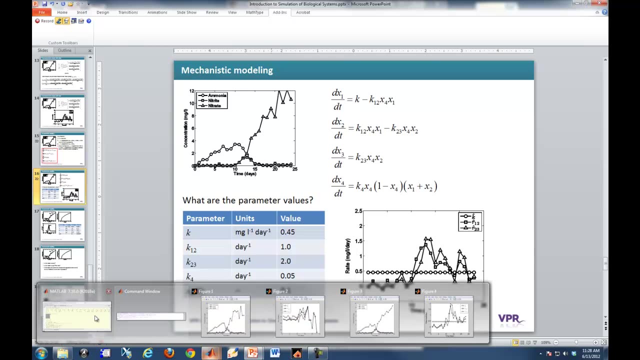 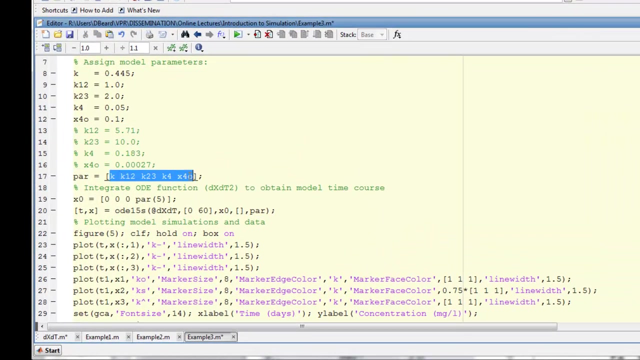 So these are our parameter values that we've guessed or estimated or guesstimated on the PowerPoint slide we were just looking at. Okay, so these numbers are these numbers here? okay, These are optimal values which we'll use later. We put those into our parameter vector. okay, 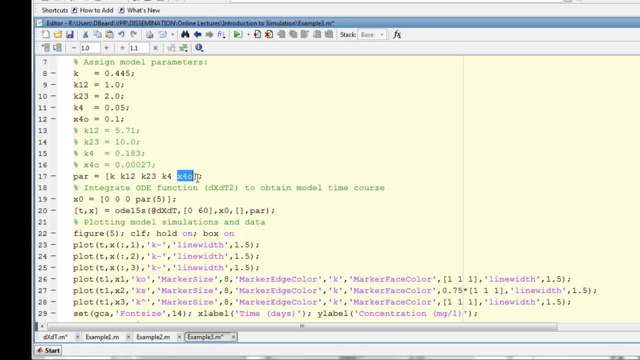 X40 is not used as a parameter in the dxdt file here, but we're treating it as an unknown parameter. We set an initial condition for our simulation. We have zero ammonia, zero nitrite, zero nitrate- but our initial condition for the bacterial population. 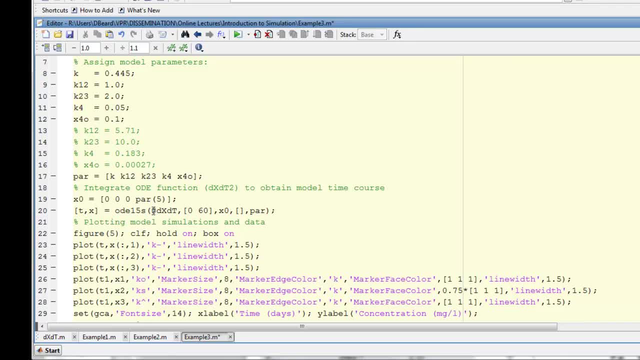 is parameter 4.. We could also just say X40,. okay, And what this command does is? it uses a MATLAB function, OD15S, which integrates the differential equation which is specified by this code here, dxdt, which we just went through. okay. 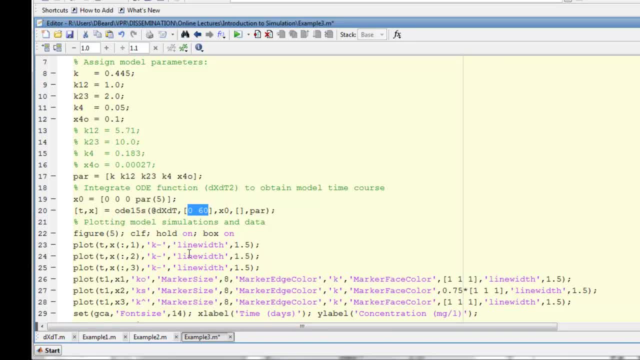 Over this interval 60 seconds. okay, I don't know why we're. let's just integrate it for 30 seconds first off, With this initial condition. this is a placeholder for some options, and then this is this extra argument: parameters: 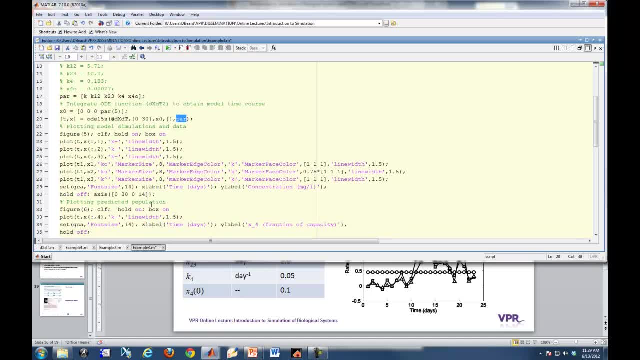 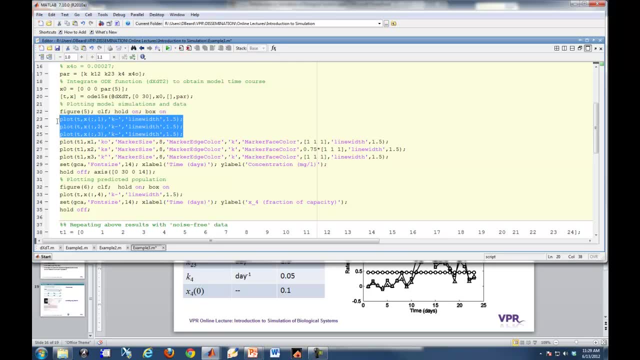 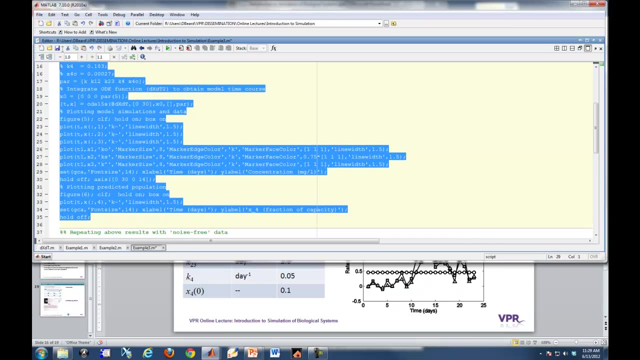 which we sent to the ODE function here. okay, And then what we do is we're plotting the raw data. oh sorry, these are the raw data and these are our model simulations, which are returned by the ODE simulation. 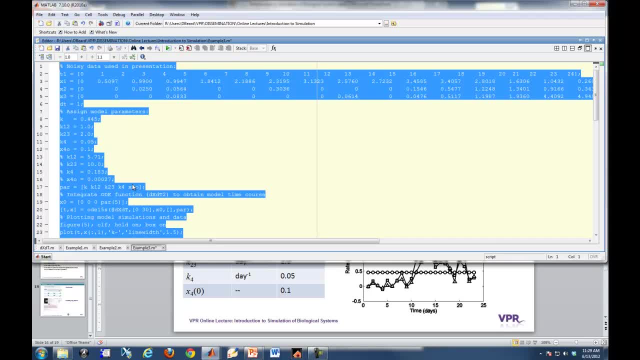 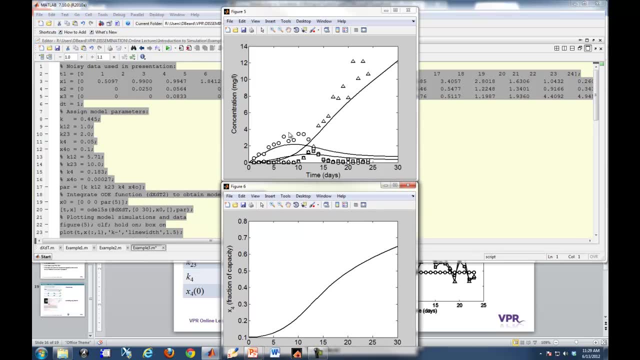 So what do we get Is executing this little piece of code. we get our simulations against the data Shown here in this figure. So what we can see is that we're not exactly perfectly capturing the behavior, but we're actually interesting. 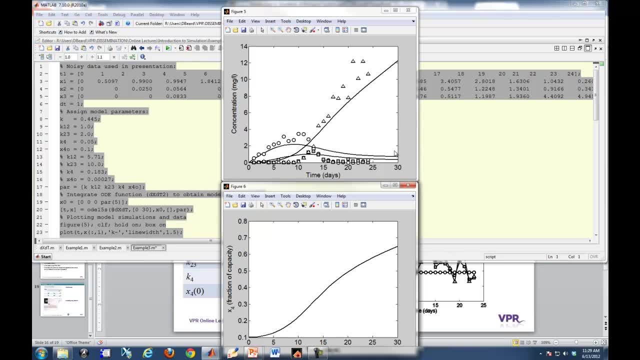 that we're getting the trends right. We're getting this buildup and then this decrease of ammonia, we're getting this buildup and then this decrease of nitrite, and then we're getting this buildup, this delayed, and then steady- sort of steady- buildup of nitrite. okay, 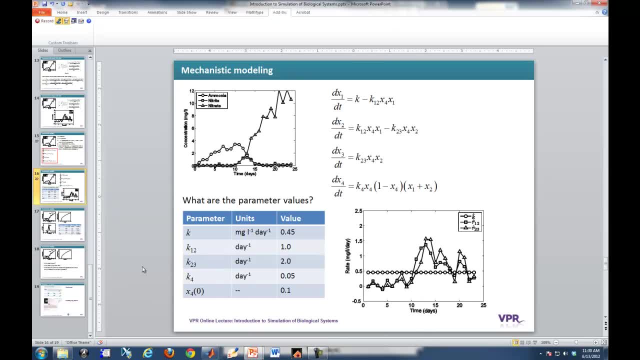 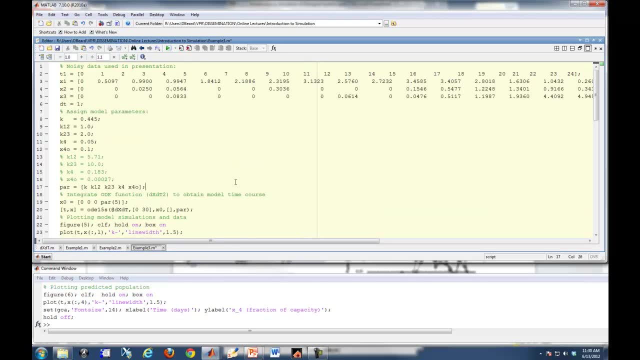 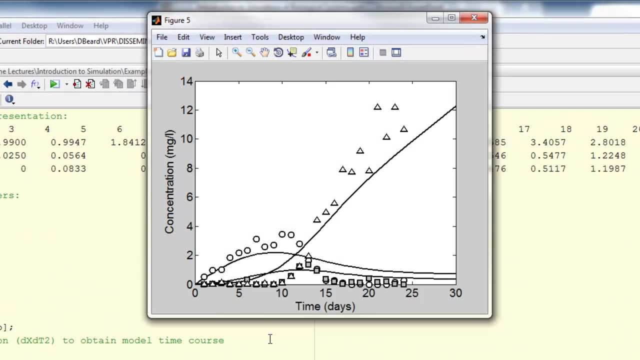 And we can look at those. well, let's just look at let's. just before we look at those, let's just go back to our MATLAB codes for a second and just tell you that. well, let's look at the figure first. 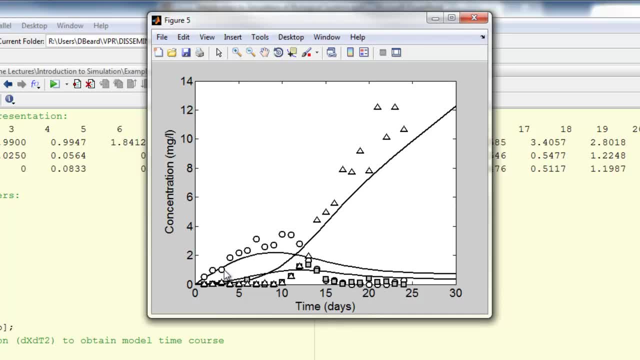 One tool that we use a lot in mathematical modeling biological systems is optimization, and that is trying to. in this case, what we can do is we can try to estimate those parameters that we guessed by trying to minimize the difference between the model predictions and the measured data. okay, 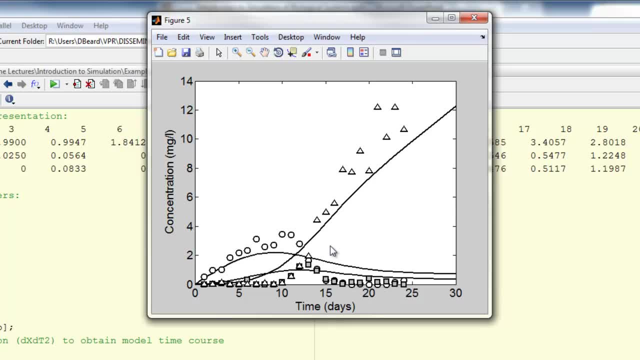 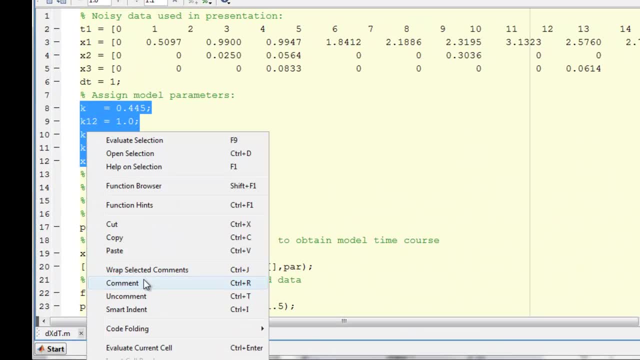 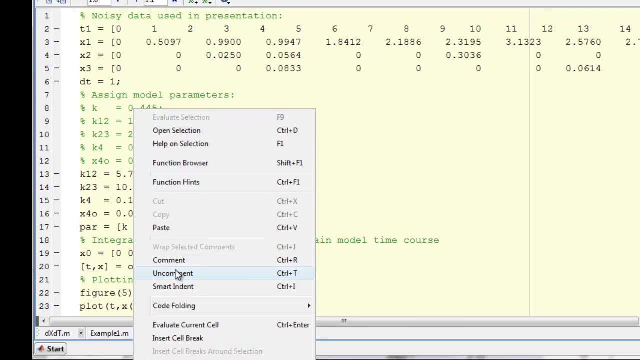 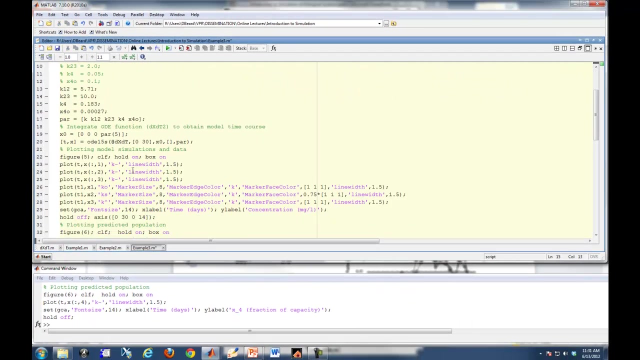 And that's actually the subject of a different lecture- how we carry out those optimization, how we carry out optimization. but what I'm just going to do is just uncomment these, these optimized parameter values here, and see that they're there, that they're different from the guessed parameter values. 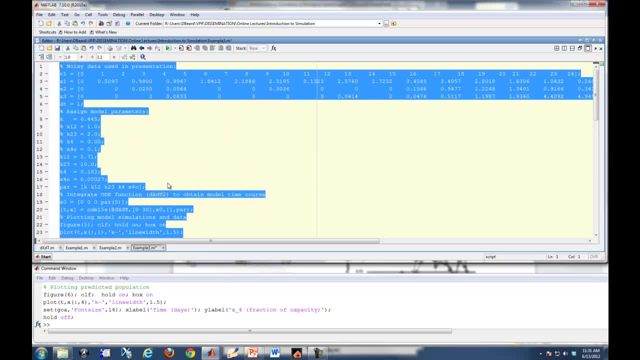 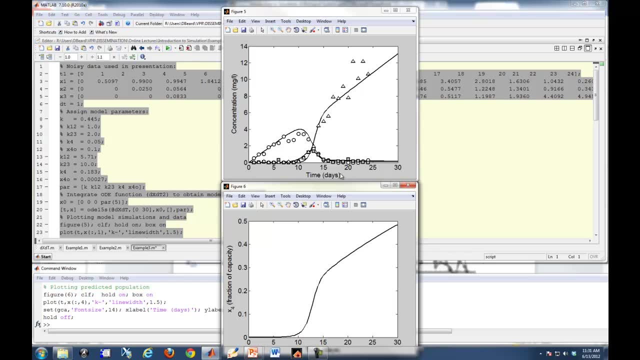 and rerun this simulation And what you can see is that by estimating those five unknown parameters, we can actually come up with a very nice fit to the data, okay, And in addition, we can then predict the X4, and, not surprisingly, this bacterial population. 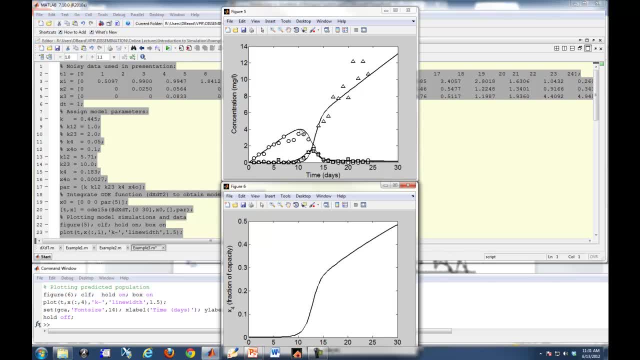 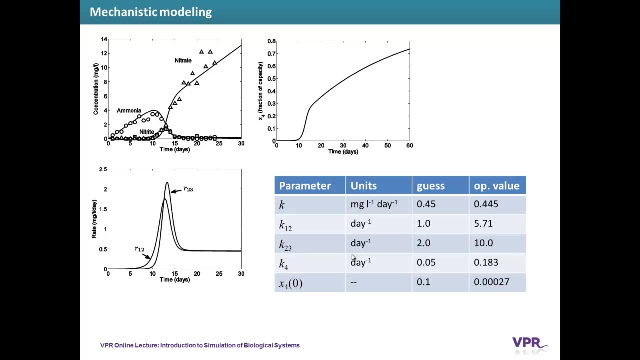 really starts to turn on and grow around to actually see consumption and conversion of these nitrogen-containing compounds. okay, So that's interesting. So let's go back to our PowerPoint here. So these are the simulations I just showed you. These are our guesstimated parameters. 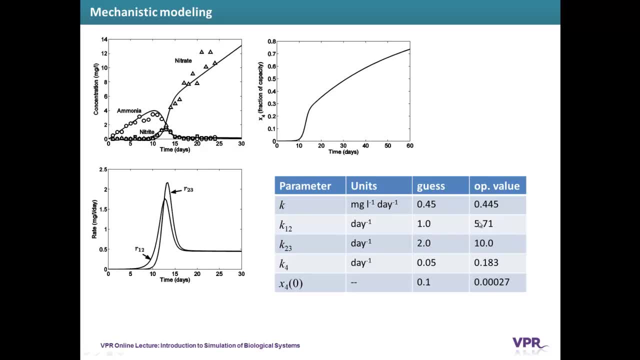 These are our optimal values. It came from some kind of optimization, of trying to match the simulations to the data. You can see that they're different Strikingly. the initial seed population is much, much smaller than one here in this case. 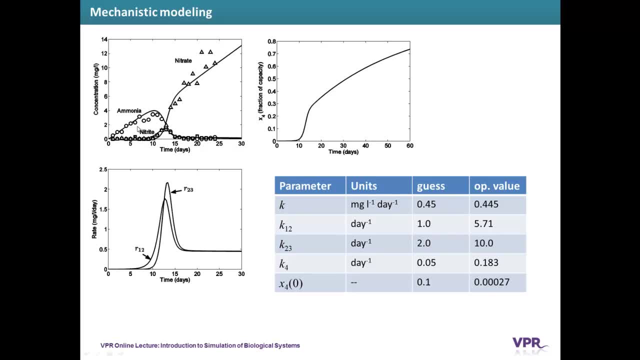 And then the interesting. the other interesting thing associated with these fits to the data is that the bacterial population is predicted- here I'm simulating for 60 seconds. it's predicted to just keep continually growing and growing, And if we simulate for longer and longer times, 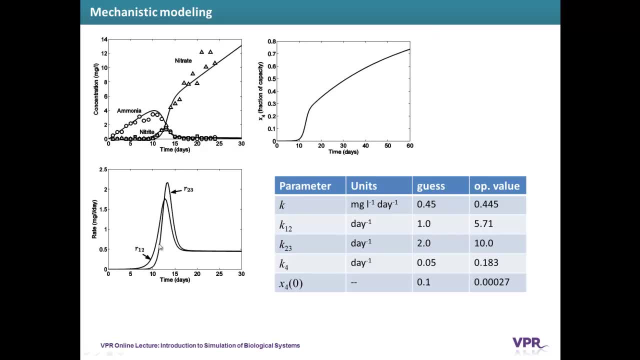 it just eventually asymptotically reaches one. So that's interesting. Our rates- R1 and R2, we can then get from the model simulations and they have the same behavior as our analyses of the noise-free data. and that is, R1 peaks around day 13,. 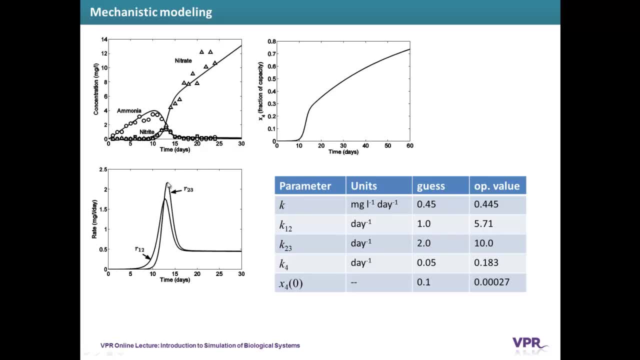 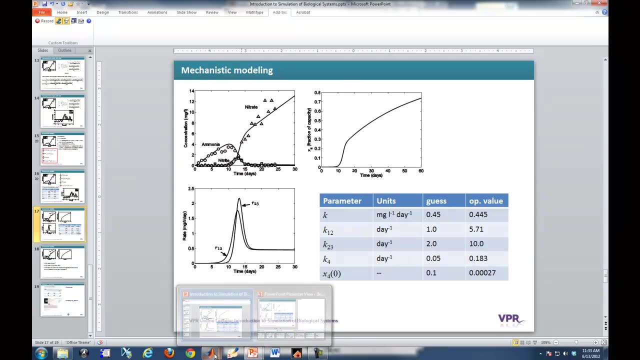 and R2,. R1-2 peaks around day 13,, R2-3 peaks a little bit later, and then they eventually drop down and converge to K, which is about 0.45,. okay, What else can we do here? 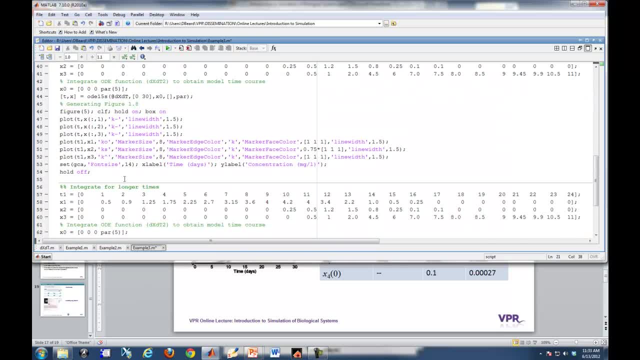 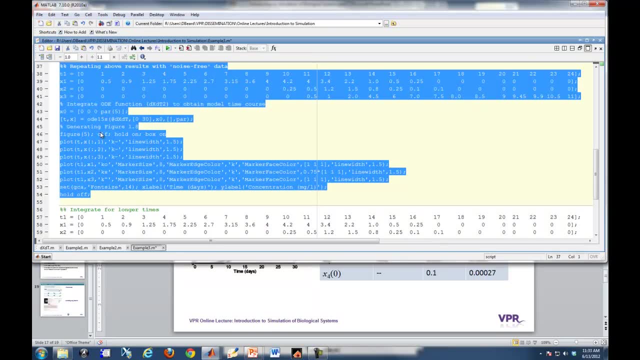 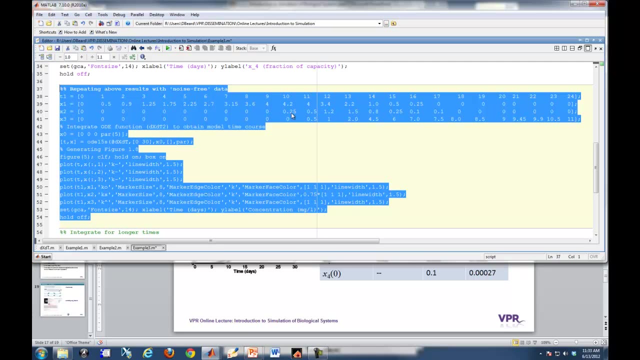 So, just to kind of wrap up this simulation, I just want to repeat those simulations with noise-free data. Okay, so this is the same sort of block of code which I just showed you, except that the data that I'm using are the initial original noise-free data set. 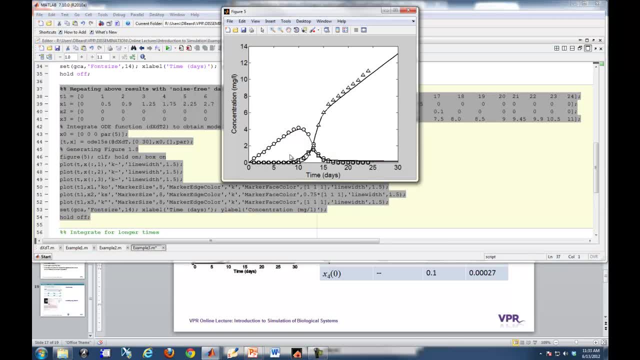 And we can see that model simulations go through the data very nicely. But what's interesting is that the noise that we saw in the previous simulation actually does a fairly nice job of masking some of the systematic differences between the data and the model. And what's particularly interesting is 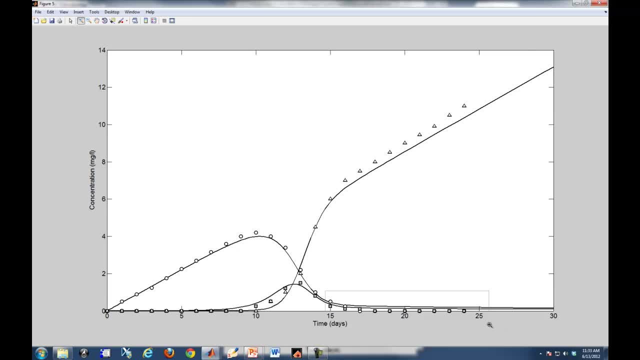 if we were to zoom in on what's going on at these times here is that the model is always predicting finite ammonia in nitrite, while our data are showing that these eventually just drop to unmeasurable levels or essentially zero. So that may be a systematic shortcoming of the model. 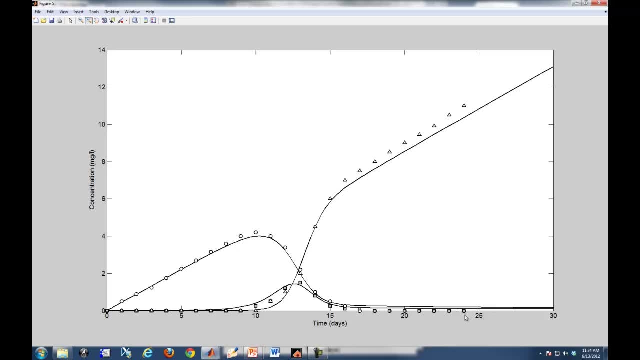 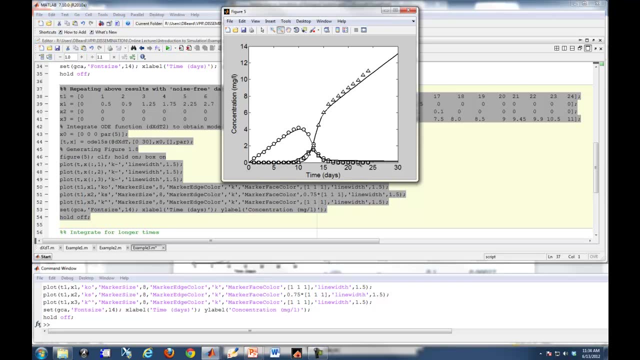 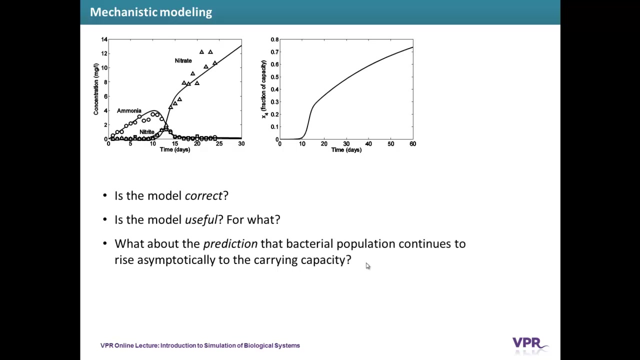 Or it actually might be a systematic shortcoming of the assay used to measure these data, because we may be just looking at concentrations that are near or lower than the limit of detection. So that's an interesting thing to consider. But just to wrap up this lecture. 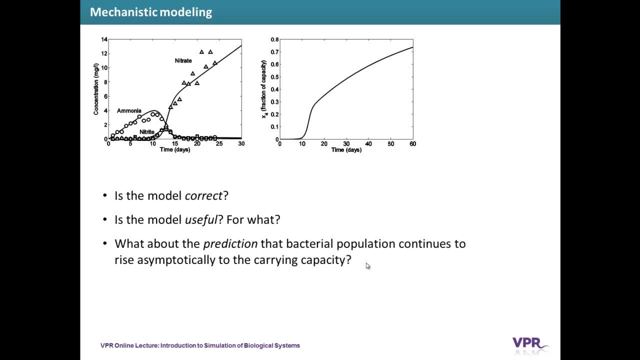 those are our model predictions against the noisy data And interesting things to consider. interesting things to think about are questions like: is the model correct? So the model is obviously a fairly crude and simplified representation of reality. You can think about some of the assumptions. 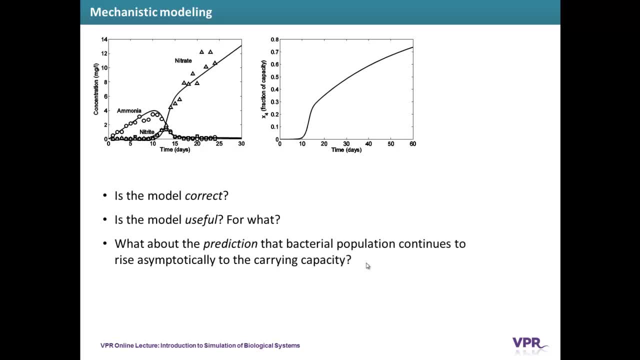 we put into this model in order to be able to capture the behavior in terms of a simple, tractable model, For example, lumping a bacterial population of nitrifying bacteria into one homogeneous population. Maybe that's an incorrect assumption. Maybe it's an adequate assumption. 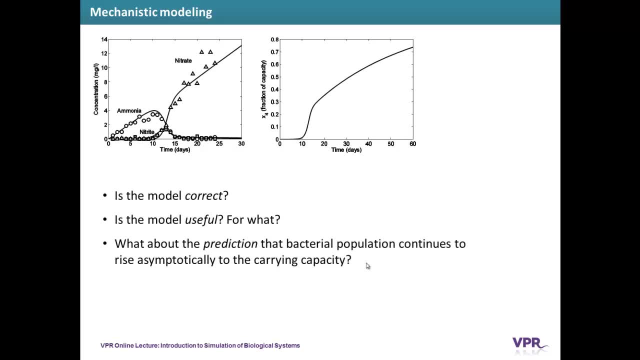 for the analysis that we did. So the answer to this question: is the model correct? Well, formally, the answer to that question is always no. No model is ever correct. The more useful question, or the more appropriate question, is: is the model useful? 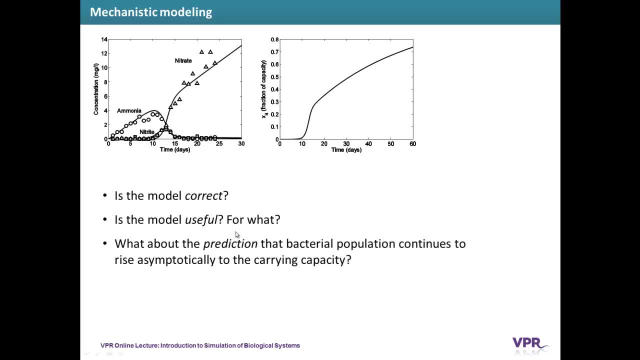 Specifically, what is the model useful for? One of the potentially interesting uses that comes out of this model is when we make a prediction about the bacterial population, And that is that it asymptotically rises to the carrying capacity And it has this interesting sigmoidal. 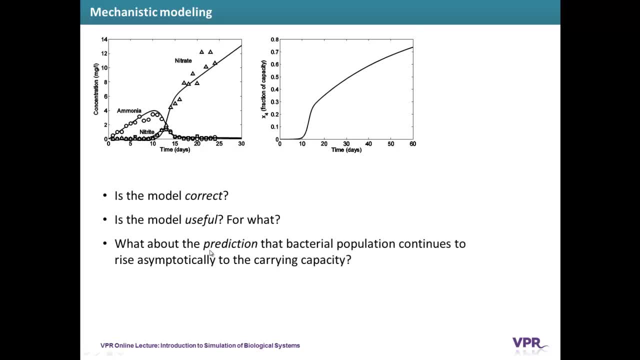 way of doing that. That's a prediction. We didn't measure that concentration, So what the model allows us to do is go out on a limb and actually make some predictions about that unmeasured variable, And then you know, maybe we could go back. 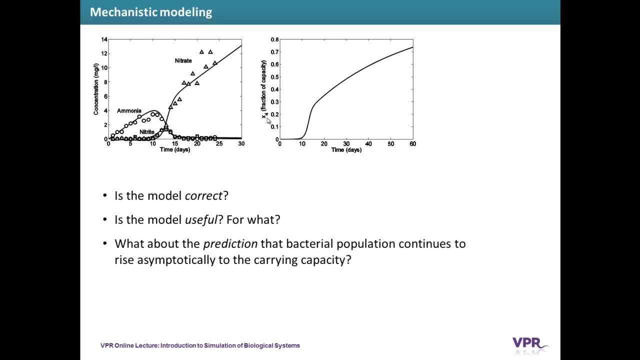 and actually make some measurements and we could test out that prediction and we could see whether the model predictions are right. And if they're right that's great. If they're wrong, then we might want to go back to the drawing board and try to reformulate the model. 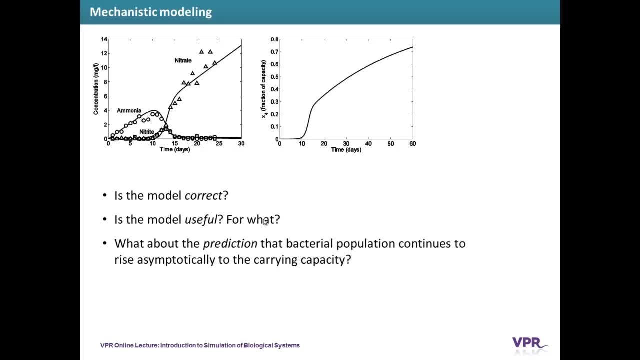 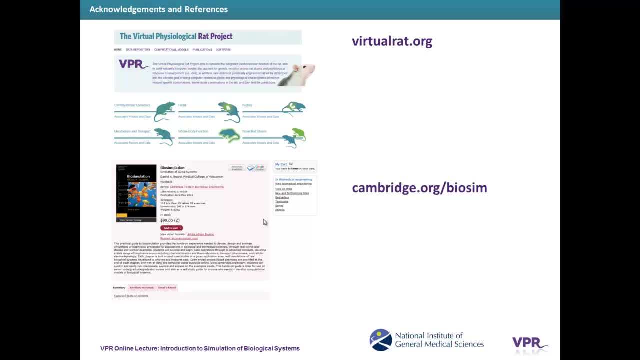 to capture additional information that we haven't put into it. So that wraps up our introductory lecture on simulation of biological systems, And I just want to remind you of where you can look for more information: virtualratorg, on the Virtual Physiological Rat Project.